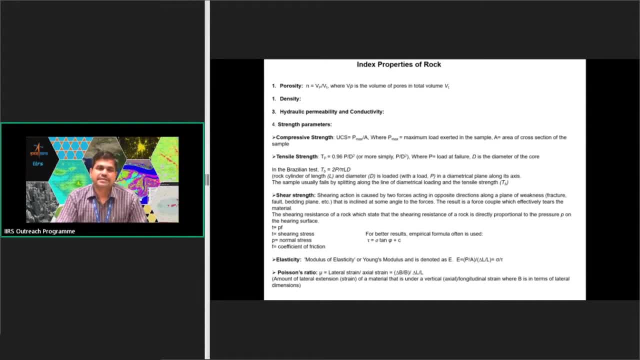 that how strong, how competent the rock is. There are three basic type of strength parameters: One is compressive, one is tensile and then shear. We'll discuss one after another, Other terms like density, then permeability, elasticity, Poisson's ratio, etc. We are not going to discuss as such because they are quite simple and has been elaborated in many textbooks. But as far as this lecture is concerned, we are going to concentrate on the strength parameters, mainly these three tensile. 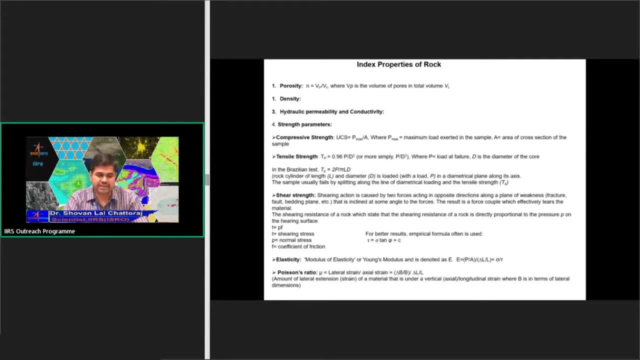 shear and compressive. So what compressive strength is? Compressive is basically: it deals with the normal load. Tensile is where you are pulling the rock mass apart, So a fracture has to develop. So that is where the load, that is where the failure happens. And if it fails, then the strength of the material has been superseded by the applied strength. We assume it like that. And then comes the shear strength. Shear strength is basically shearing. action has to take place, Shear by what we 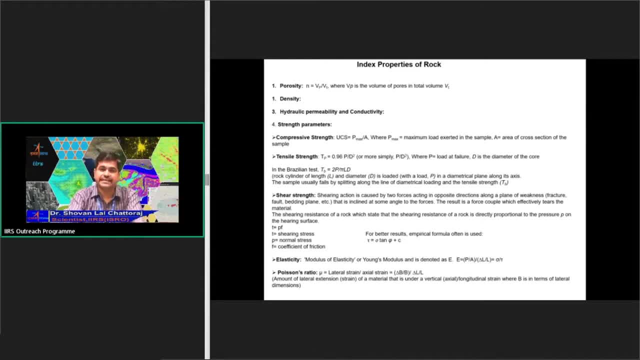 mean by shearing. Shearing is caused by two forces acting in opposite directions, So the materials they shear past each other. Once they do so, the shear failure happens, And this is the main cause. because of this, only the landslides keep on happening. So shear failure has to happen. Shear strength has to be more than the applied strain, so that if the strength is more strength of the rock. 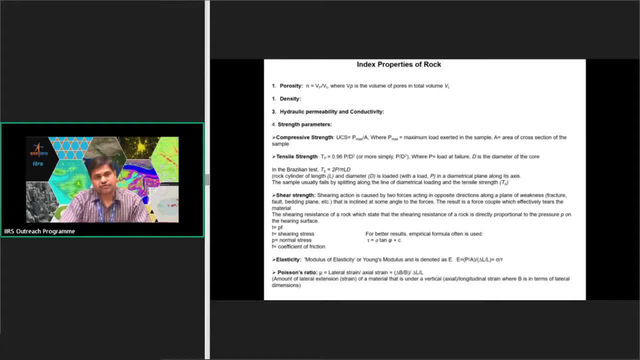 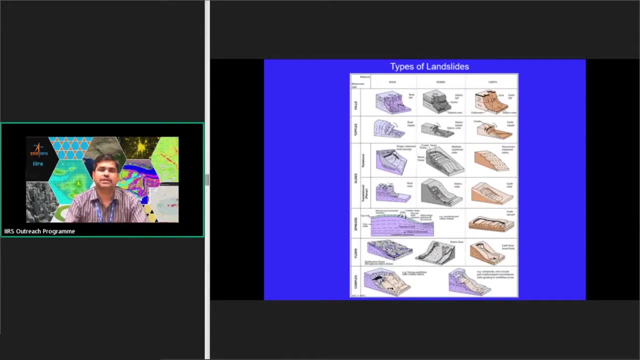 the material is more, then it will sustain. If the stress is more, stress is more than the strength of the material, then the failure will happen. Shear failure will happen, followed by the landslide. So we'll move to the next slide where, directly, we're going to jump onto the types of landslide. What are the different varieties of landslides? So if you see this chart that takes me, this photograph tells that there are two axes of landslide classification. 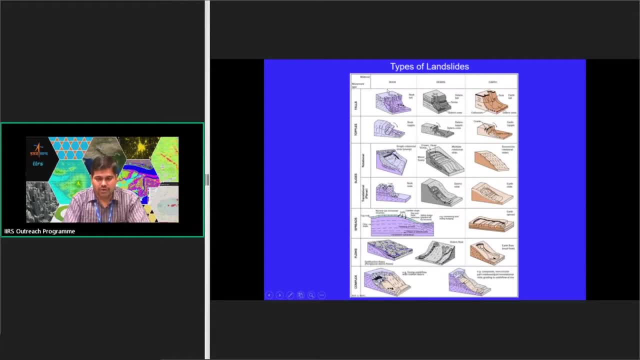 In one axis we deal with the different type of material involved, like rock, debris or earth, And this axis tells us about the processes involved. So it can be simple: rock as a material, and then rock may simply fall, falling apart of rock, then the debris in between and earth. Earth is nothing but soil or clay material. So debris is a mixture of all this, So it's a rock chunk basically embedded in. 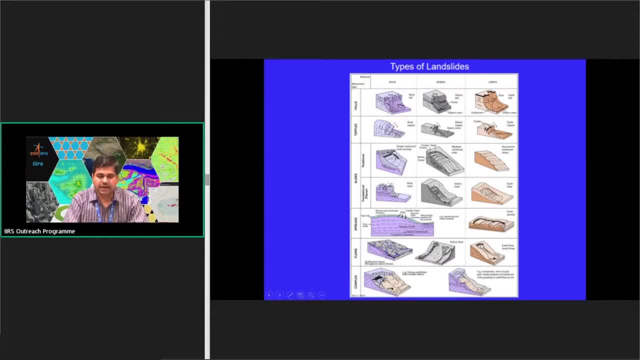 debris material embedded in clay material And rock as such is your intact rock. So the rock can fall, debris can fall and earth can also fall. But obviously the chances of earth fall is quite less compared to rock fall, where a solid thing has to fall. Then comes topple. So toppling the difference between there's a difference between simple fall and a topple. Topple has to happen along the discontinuity plane. It can be a joint plane, can be a fault plane. 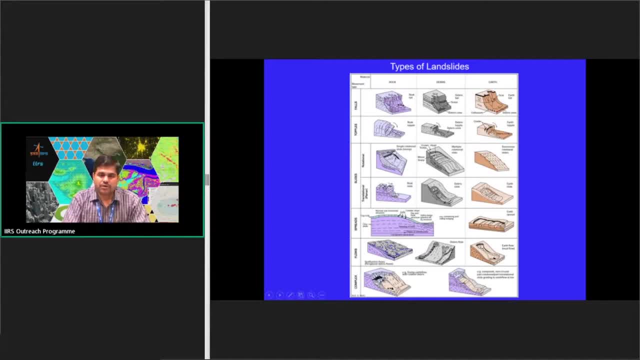 It can be other type of discontinuities. So along that discontinuity the whole material, one slice of the rock, is basically falling, So that we call topple. So it can happen that rock will topple or a debris will topple or earth will topple. So obviously, again, the rock topples are more prominent, more apparent compared to other two varieties. Then comes my typical slides. Please understand that we call, very often call. 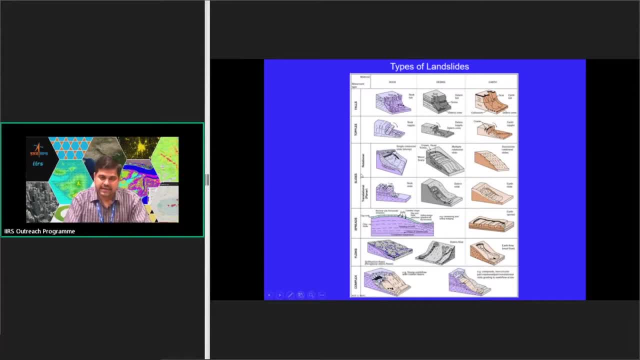 landslide. But this term landslide is coming only here. Slide Slide can be rotational, can be translational. Rotational is where you know shear plate is a curve, So there's a rotational failure And the failure can be simple: rock slide, can be debris slide, can be earth slide. Similarly it can be planar also. So planar rock slide, planar, debris slide or earth slide. So slide constitutes of rotational and planar failures. Then comes my spraids. 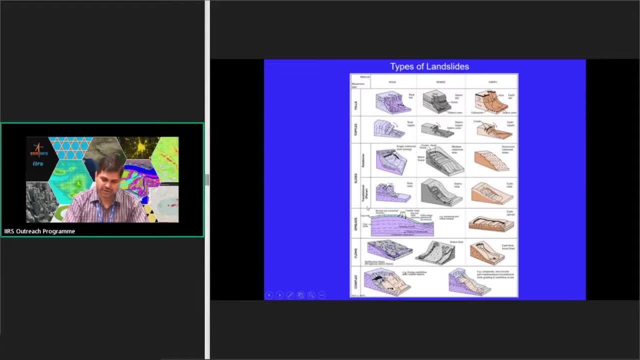 Basically one thing we have to take into account that if I go this way, if I come down, then the water content in this different types of failures are continuously increasing. If that increases up to this, up to slide, we can think of that. it was quite dry material was involved, obviously aided or triggered by water, But this spraid onwards, the material is intricately mixed with water so that the whole material is it. often it becomes a slurry kind of thing or a spraid kind of thing. 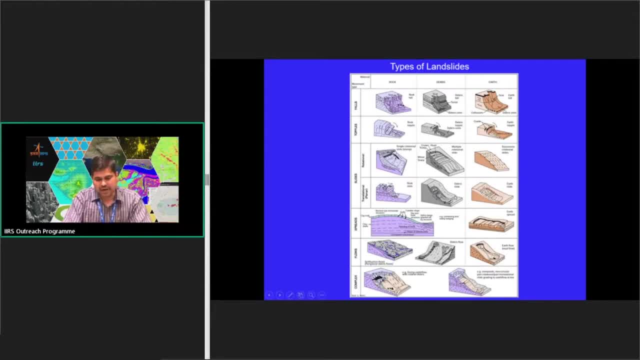 So rock and debris, we club it together and then earth spraid, Please mind it. The moment I crawl I increase the water quantity, Varieties of this, the variety of slides occurring here. they are more in number because rock as such a solid material now will not spraid, but earth, because it's clay mostly, it can very well, very easily spraid. 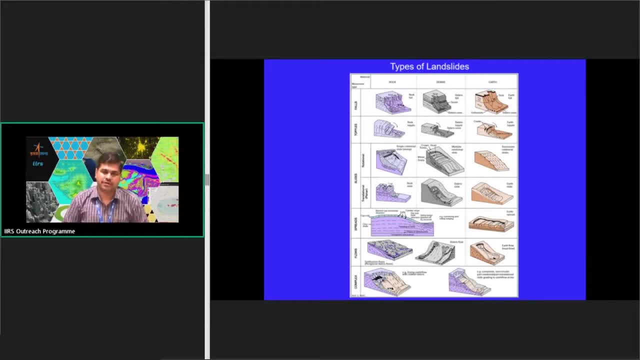 Then comes flow. Flow is obviously when water quantity, inherent water quantity, is sufficiently large. uh, so main part, main contributor, will be from mud flow or earth flow. then comes my complex. complex is a mixture. it's a variety of all kinds of you know. it can be fall plus light, or can be supposed top root plus spreads, anything it can be. 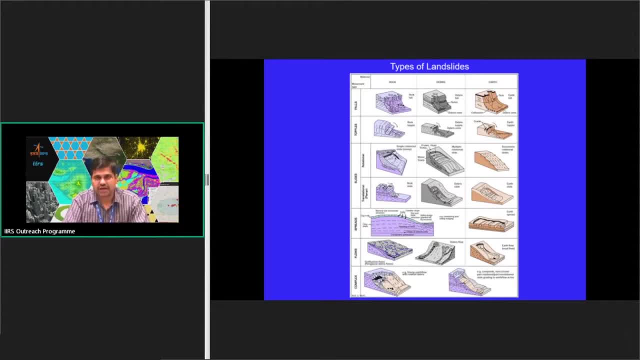 so any big landslide. normally it happens so that it's not a peculiar particular type of plants, right one type of plants, rather it's a mixture of uh, one or two. so when it is a mixture it's very easy to um think that you know the top portion, where the source portion, basically where. 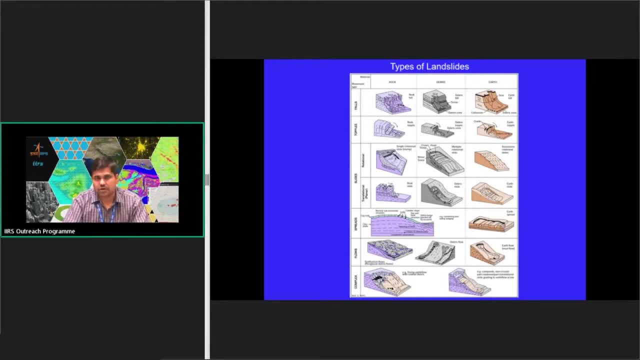 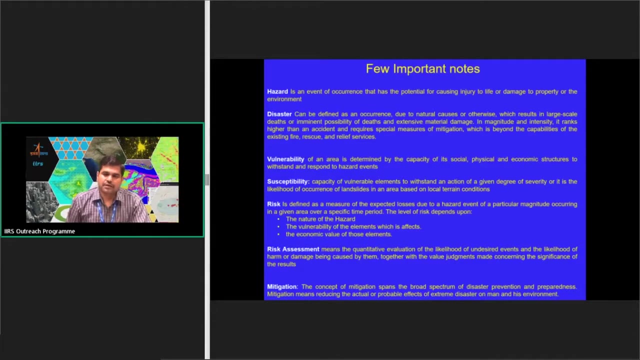 from the material is coming, uh, that can be a simple rock topple or rock slide, and then, as it goes downward, uh, towards the valley, it may become, you know, may take a shape of a spread or a flow. normally it happens like that. then comes three important notes that we need to uh uh understand. hazard: what is that? it's an. 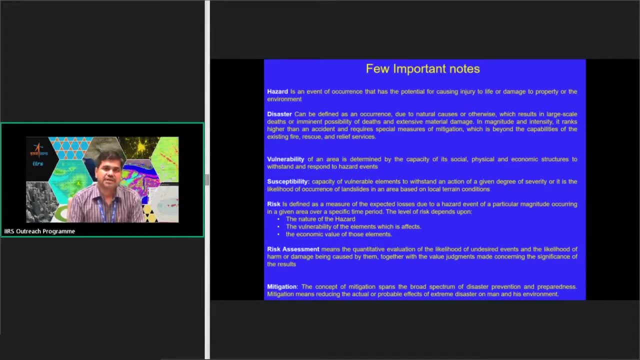 event of occurrence that has, you know the, the potentiality for causing injury, life, uh, or damage the property. so that's hazard and disaster as such can be defined as occurrence, different natural causes or otherwise, but large scale, uh, dates or imminent possibility of death, etc, etc. so hazard and different, hazard and disaster: there is a difference now i 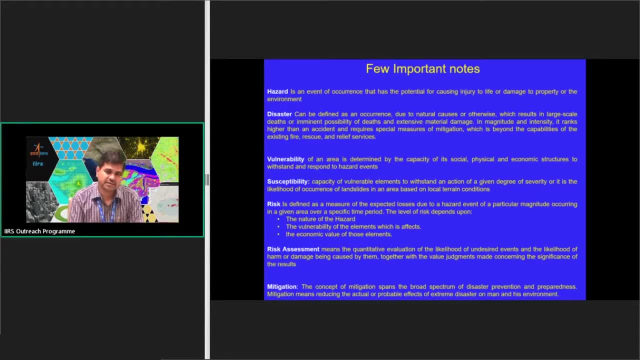 come to the main three uh units, main three definitions that we should learn: vulnerability, susceptibility and risk, because any kind of you know, disaster study, uh, let us take the landslide as such. we have to, we have to define a landslide in terms of its vulnerability, susceptibility and risk. so what vulnerability is it's an uh, it is basically areas, sorry, element specific. so 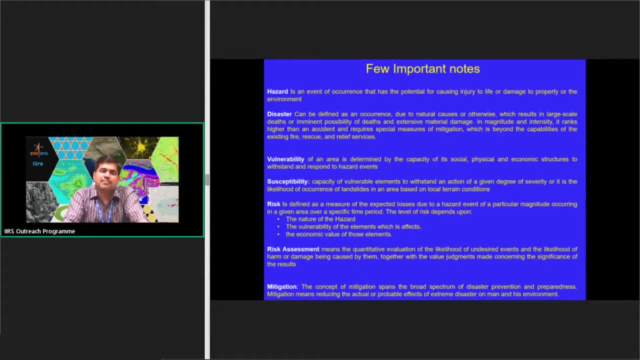 element specific means i have to have vulnerable elements present in that landslide prone area. so what do i mean by elements? elements can be simply, uh, the population, human population can be cattle, shed can be my roads, can be school buildings, normal buildings. so all these are they are, they remain at stake when a landslide hazard um is being considered. that's why the elements are. 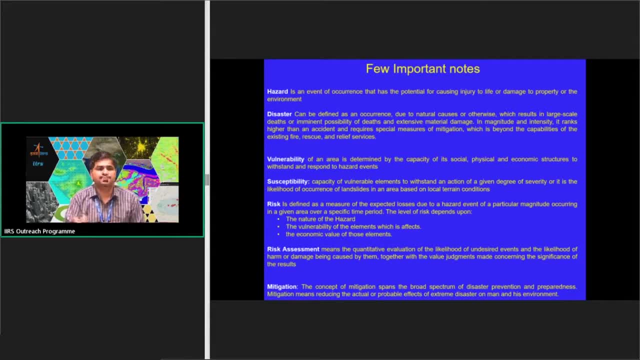 at uh stake. so this increases my vulnerability. so simply, vulnerability is dependent upon the elements present. if there is no vulnerable element present, the vulnerability of that for that particular type of register may be close to zero. then come to susceptibility. what susceptibility is? susceptibility is simply: it deals with how much sustainable that particular land piece is. obviously, 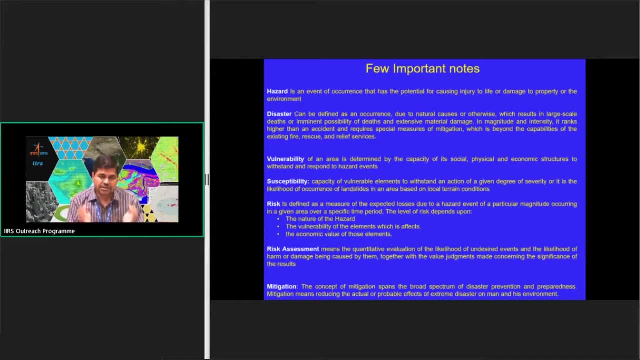 you know, in a fixed time ratio, time domain, how much sustainable that land piece is for a particular type of hazard. let us take a landslide, let us take a flood, for landslide to take place in that area, how much sustainable that area is. what, basically, are the factors for determining sustainability of an area? the factors should be: 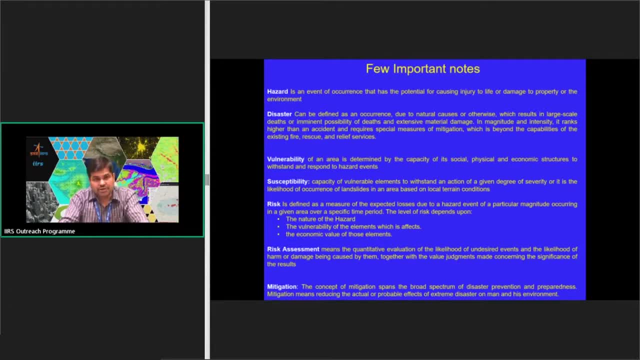 can be geological, can be geophological, can be seismological, whether no R squares keep on happening in that area or no, or what is the main rock type of that area? what is the soil cover? how much the area is, how much proximity with major fault system, or suppose how much distance the 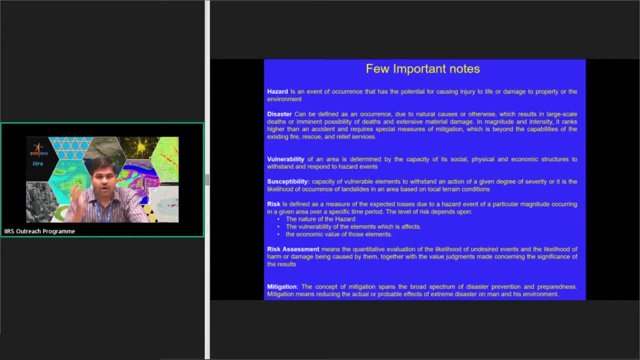 area is from your major river and drainage network. so all these contribute to uh calculation of sustainability. so all these basically makes the area sustainable. if uh no area is free from this kind of sustainability, obviously the overall sustainability of that area because of that particular uh type of hazard. let us take 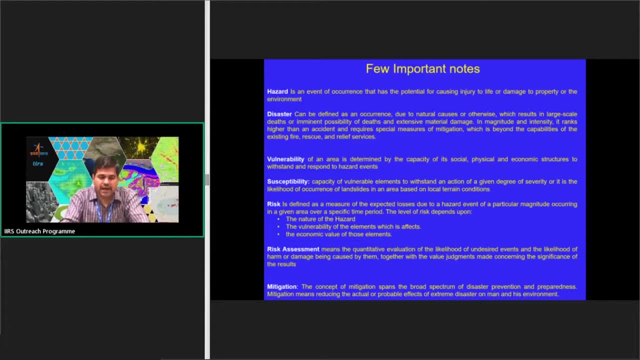 landslide is close to zero. the risk, on the other hand, is basically, it takes care of both vulnerability and sustainability. so, if I are, if I want to calculate the risk of an area because of a suppose hazard, uh, we have to consider vulnerability and sustainability. apart from that, we have to take 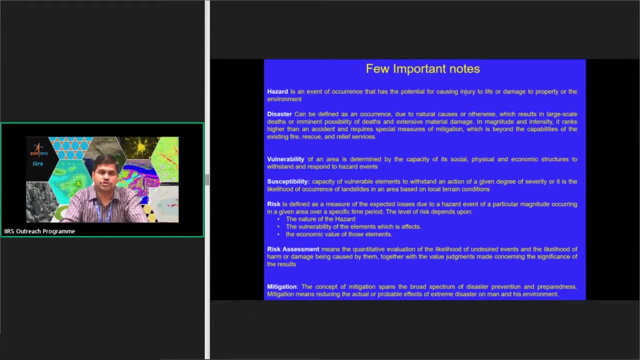 exposure. also we have to, you know, get to know about the socio-economical constitution of that area, or if I, if I keep this apart. so my main two technical themes will be vulnerability and sustainability. so risk I can define is a is a product of vulnerability into sustainability. so 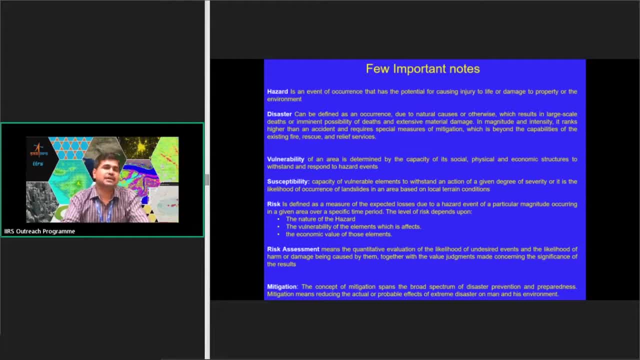 if we take an example where your suppose vulnerability is quite less, that means there is no element somewhere, in suppose in hilly state. like there are no, I mean very less elements so very less population, suppose cattle shed or villages. so my elements are less, so that makes my vulnerability, uh, quite low, but at the same. 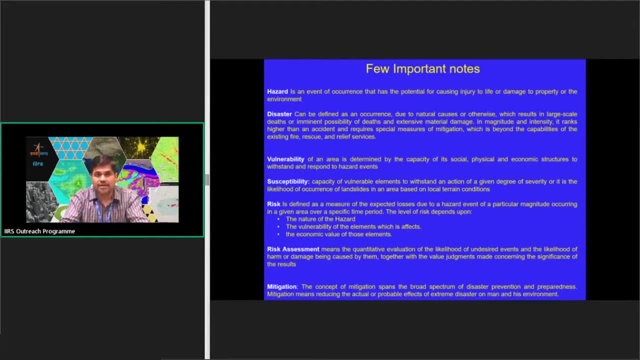 time. that is, you know, on the lap of Himalaya, so every now and then that is being shaken, uh, like anything, by earthquakes. so it makes the area sustainable. so sustainability may be close to zero and vulnerability may be close to. um, vulnerability may be close to zero, sustainability. 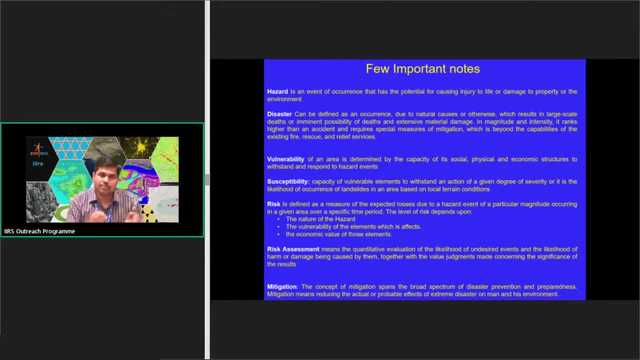 may be close to 100.. so from this 100, 0 to 0, 100, all possibilities are possible. let us take an example from, suppose, one plane city, like you know, in in somewhere in Indogangetic plane landslides may not happen there, but that is highly populated, densely populated, so that makes elements present. so 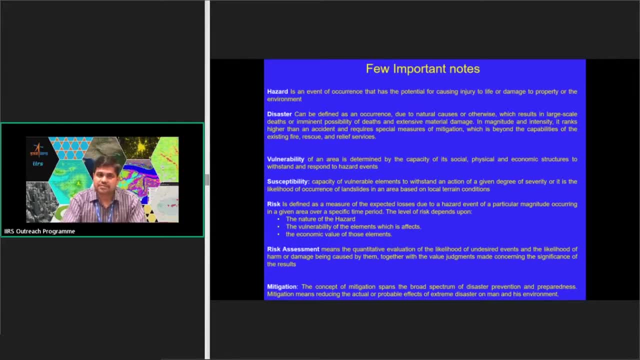 if elements are present, vulnerability is high, but it's not sustainable. so it is not sustainable. the sustainability will be close to zero. vulnerability is 100.. so, as I have told, it can range from 0, 100 to 100 within this road range, anywhere your risk may lie. then come the risk assessment, if you have. 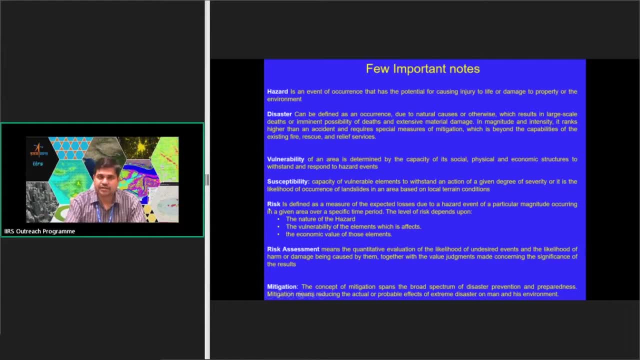 um well assessed your vulnerability and stability and risk. you can assess the, you can go for the risk assessment also and mitigation is the last thing that you can do. uh, for mitigation we have I have some slides that you know. I will discuss how to you know better mitigate a landslide hazard. 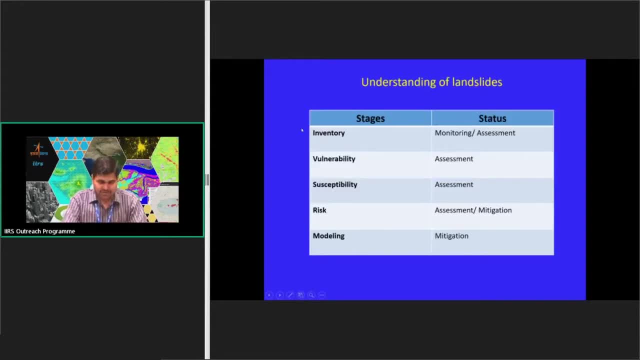 now different stages of landslides. so fast, start from inventory thing. inventory is nothing but making a landslide polygons on a, a repository kind of thing, suppose on a satellite image or any other uh platform. so inventories are those polygons will which will tell you where uh the landslide is taking claim taking place. so it. 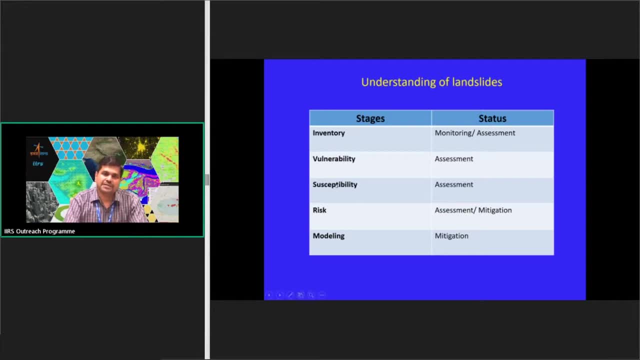 is basically a monitoring on an assessment thing. then comes the vulnerability and sensitivity, as we have discussed. they are again assessment, but risk is, if we have calculated the risk, that means I am or we are already on to mitigation. and then modeling: modeling of a landslide for a better characterization. 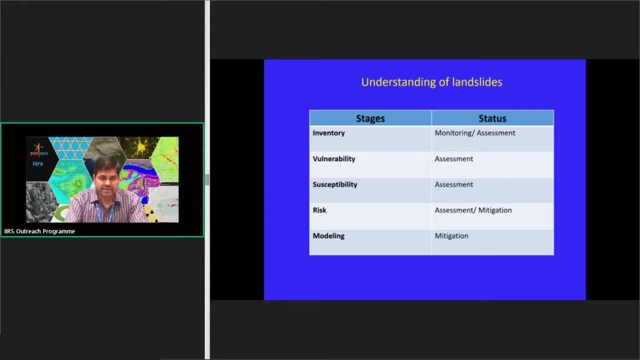 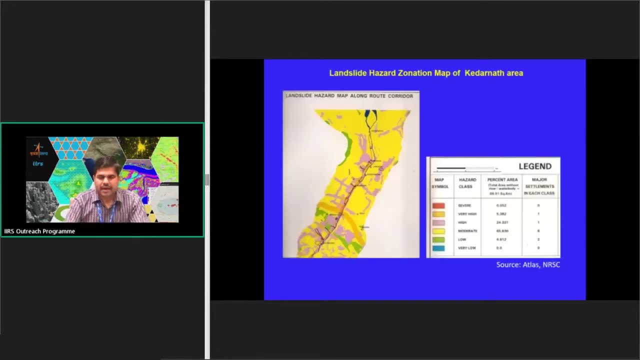 for a futuristic prediction. so they are totally dedicated to mitigation. this is a map that has been developed by Indian Institute of remote sensing. this is in a part of NRC. they have come up with a nice map where you know you can see different colors. these colors indicates different. 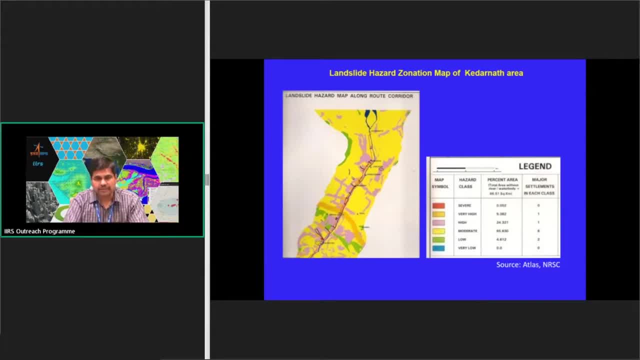 yeah, yeah, select these regions as well also are very um. so this is a a town called ketan that was devastated. if you uh, well, ever about which sites? its really pretty low in number. so we have taken that is the blue one, but it indicates very low theyadel, sozusagen. so total my 36 classes. that's all the six classes are there. So all these six classes. with these six classes, I can tell which part of the land piece belongs to how much hazard, hazard potential. So this is a town called Kedana. people are aware about the tourism authorities and, muy far at Manila, san painting планet, but this is the same area called Kidanthat. it is dist, mr Modesto. so if you are aware of more about those plans, then go to kidan dynamics. the rest of the class has indeed learned this course. 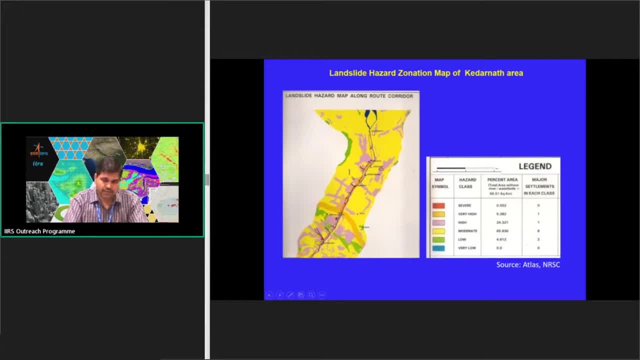 it in 2013 flood event. so please see that all green areas surrounded by this already indicate they are. they were in very high uh landslide hazard zone, so they were already inside the hazard zones and this was people prepared quite, quite ago before uh. then your 2013 event somewhere. 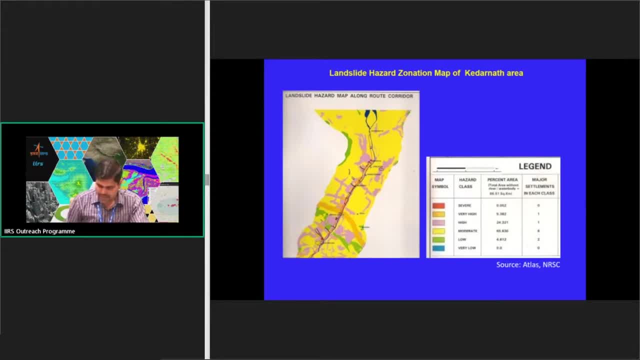 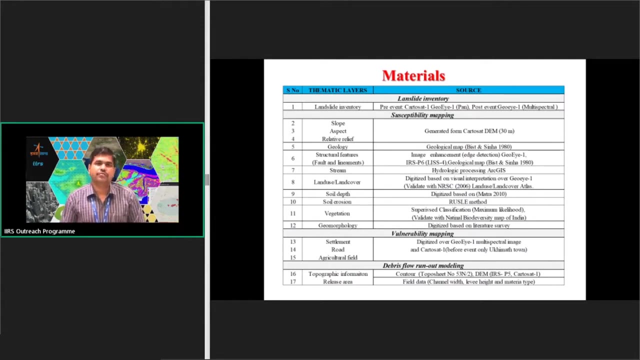 in early 2000. this was prepared. from then onwards, it was known that this zone belongs to a very high to severe class. now comes we have discussed about, you know what, uh, the definitions of vulnerability, susceptibility, risk, and you know how to, you know, define this, how to detect a risk. 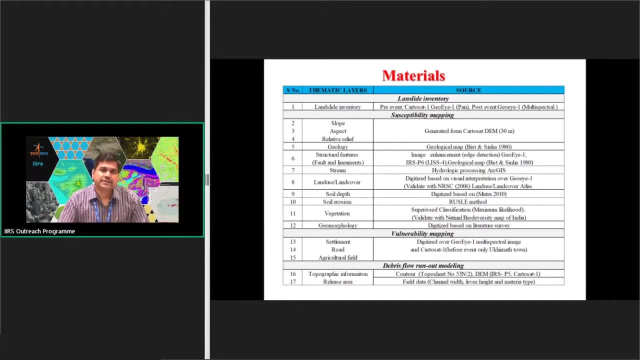 hazard, suppose, for detection of a risk hazard, i need my vulnerability to be calculated, I need my surstability, etc. Now, how do I do that? So the basic methodology. for the basic methodology, if I want to discuss, I need some kind of materials. 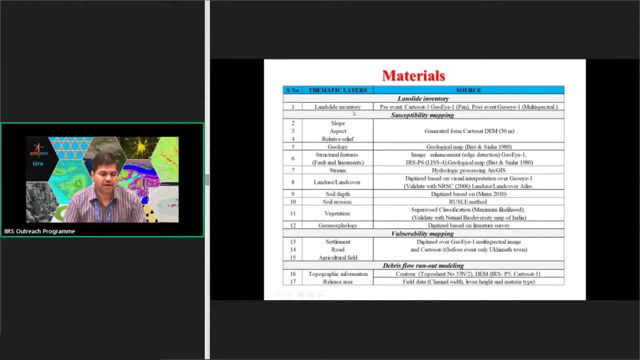 What are the materials? Please look at this table, where you will find that I have to start with a landslide inventory. Inventory means it's simply a repository of the polygons where I know that this sure-sort landslide is happening. So an inventory basically can be made from normally freely available open source satellite. 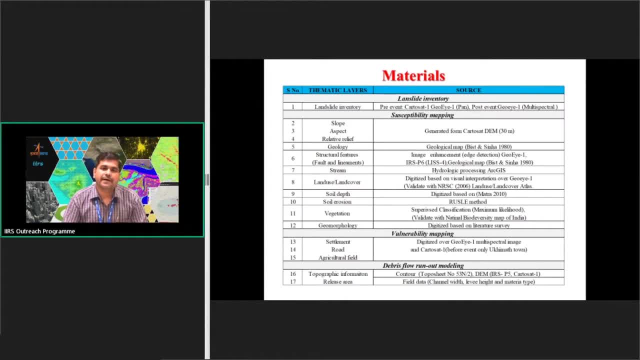 data or maybe available from, can be made from the procured data, also Even people. they can try building their inventory map from simple Google Earth images, the images available at Google Earth platform. From that also they can create their own inventory. So it's the need of making an inventory I'll discuss later. 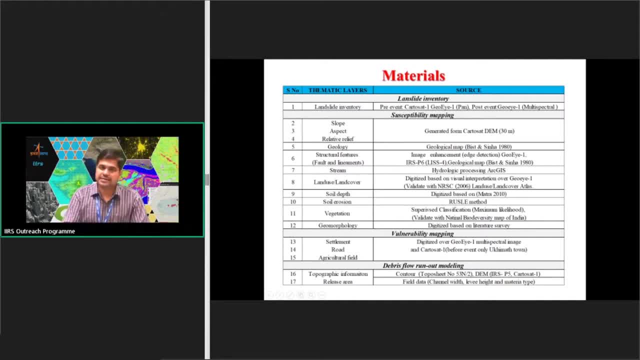 Let us understand: what do I need for Bhalva? So for Bhalva it's mainly element specific. That means I have to map those elements. What are the elements? Maybe villages, maybe cattle sets, maybe roads, So all these things. 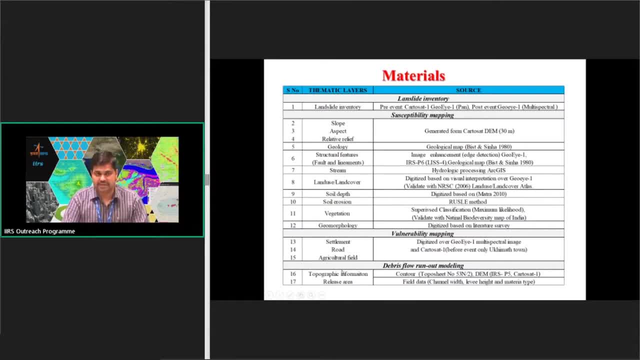 Here we have taken the settlement road and the agricultural field. We have to map this Once, we map that and then weigh them. I think that among three, among these three, I feel the road is the more is that more vulnerable, is more vulnerable. 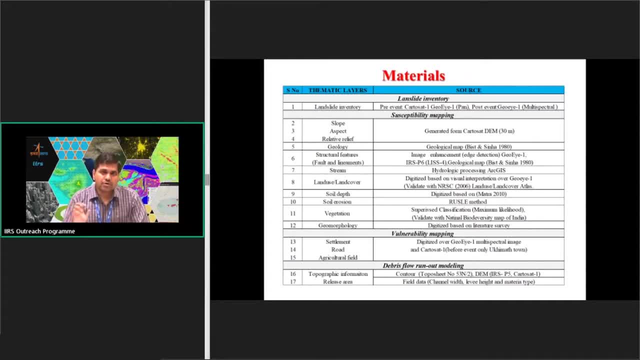 So that makes my road more vulnerable, So that makes my road more vulnerable, So that makes my road more vulnerable. So I can assume that, if I assume that I will give more weightage to that, So likewise, suppose settlement, I think, is the least vulnerable element. 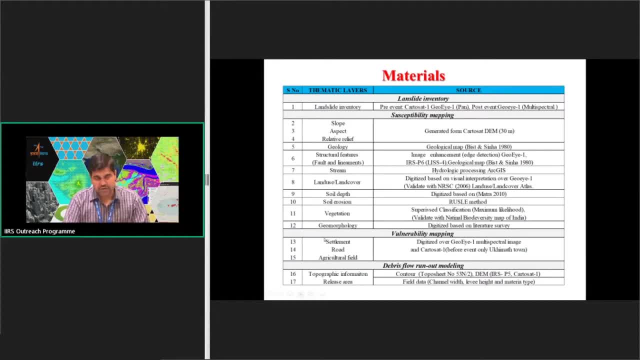 It can happen, so You can further weigh, when give weight, to give weights to these three elements and then come up with maps: Raster map For sustainability mapping we need. on the other hand, there is 12 classes, suppose 10. 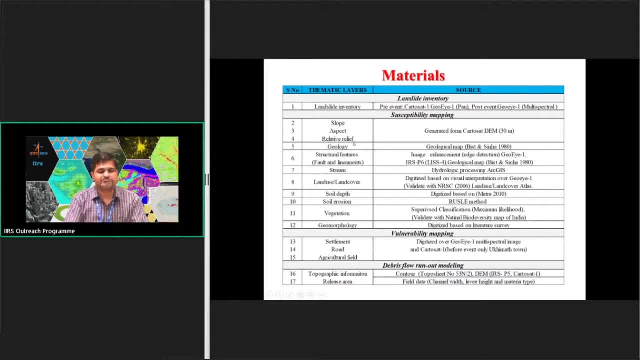 number of thematic layers, So slope aspect, relative relief, geology, structure stream, land use, land cover, soil depth, erosion, then vegetation, geopolitics, all these layers, So they are called each one thematic layers. 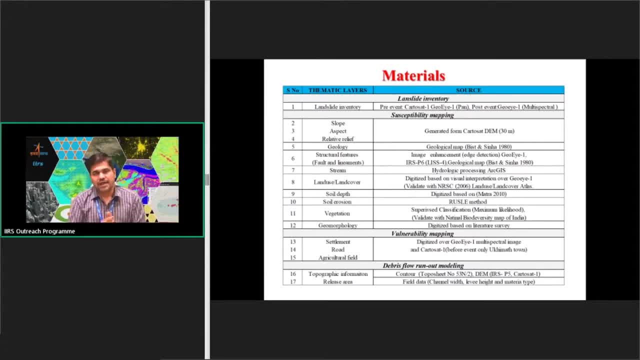 So if I stack these layers one after another and then if I compare these with my earlier built infantry map, I can readily have an idea about where the landslide is happening. Suppose we take a thematic layer, the first one, that is, slope. 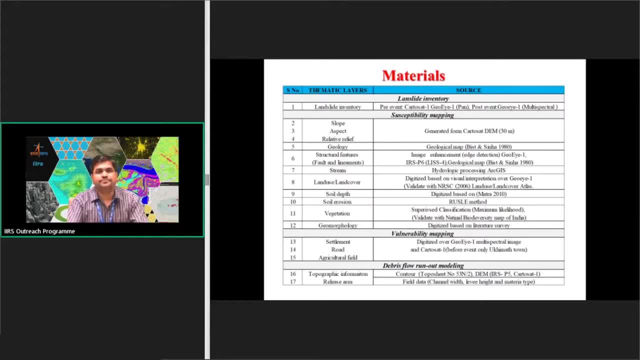 So slope is a thematic layer. In this thematic layer there will be, suppose, four classes, So 0 to 30 degree, 30 to suppose 45 degree, 45 to 60 degree and 60 to 90 degree. 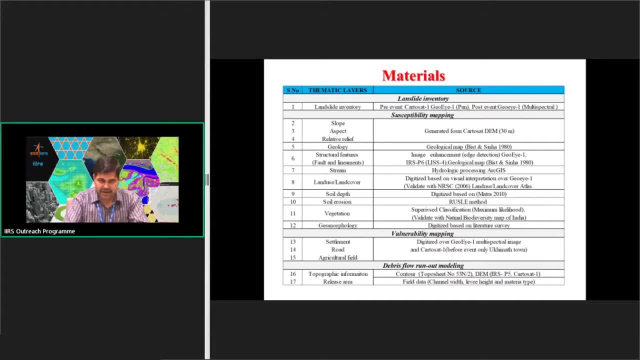 These four classes I have come up with. So the whole area, the study area, is divided into these four classes. If I juxtapose my infantry map on this slope map, what do I see? I see in which type of classes Among these four classes. which type of classes the landslide polygons are falling. 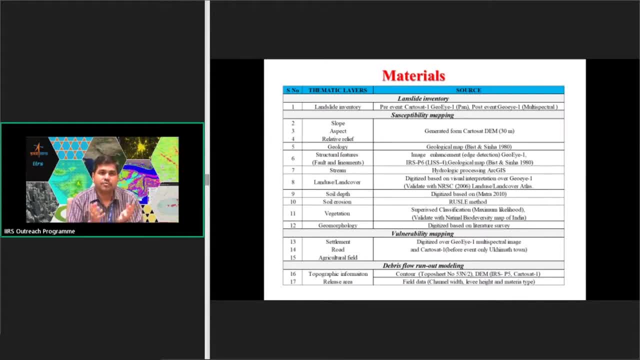 So landslide occur. landslide occurrence is maximum. in which type of slope? So if I combine this map, this information is going to come out. Similarly, if I combine the infantry map with suppose geology, I mean with suppose rock type- 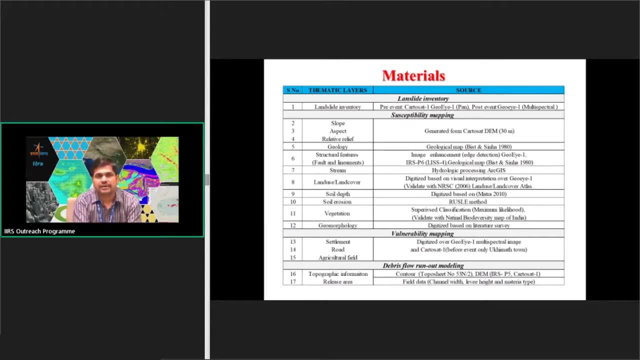 So that will tell me that which type of rock side is responsible for Landslides to happen. The class which will contain more number of landslide polygons from the infantry map will tell me that. okay, this particular class is responsible. 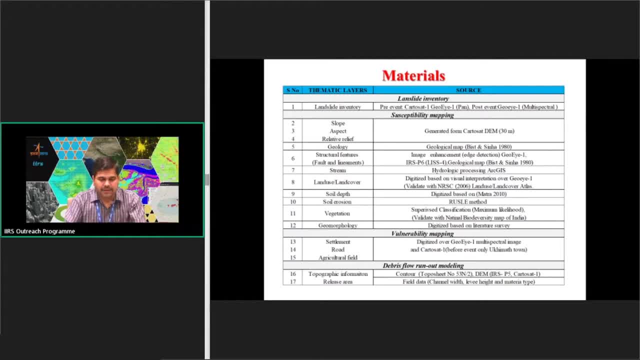 And this is less influential like that. So, likewise, what I do, I cross the infantry. That is the beauty of the infantry. I started with that infantry map, with each of these sources, each of these thematic layers. Each thematic layer consists of classes. 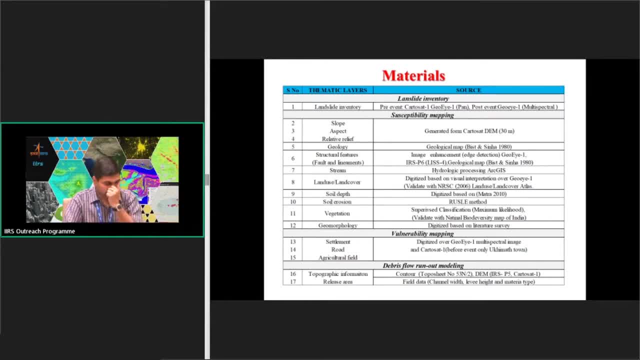 So There will be distribution, There will be final map if I get it like that: I have crossed infantry with slope, I have crossed infantry with aspect, with relative relief, like that, And the one-one combined map I have prepared. So if I join, if I stitch this combined map again and build a simple map, one map from these 12 maps, 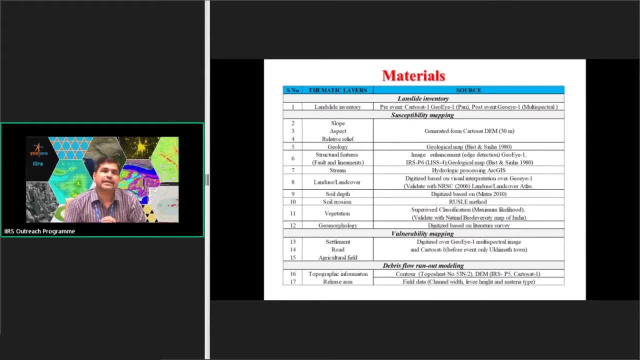 that will be my sustainability map. Here also I can give some weights, If I think, if I am well, If I am well aware of the area. I think that no geology is, most you know cause, the most influential factor for all kinds of landslides in that area. 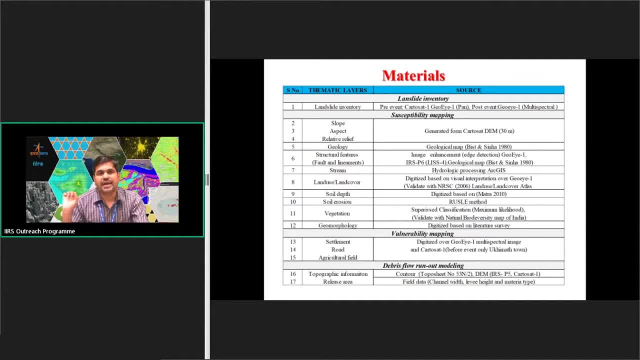 So I will give, while stitching, I will give geology maximum weightage. So by now I hope I am clear that what I have done, I have made an inventory, The inventory map I am comparing, I am juxtaposing with each of the thematic layers, slope to geophology, suppose. 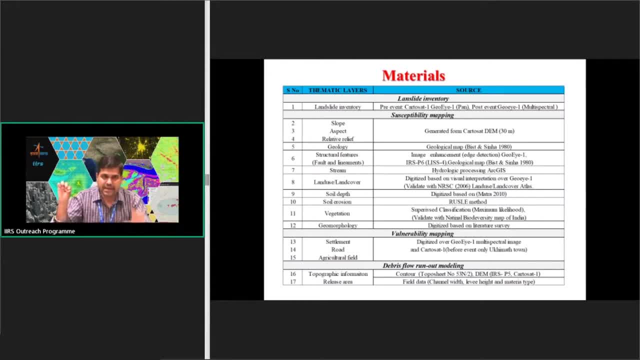 And I get a combined map. Now, From each of these two I get one-one combined maps. So I have total, suppose, 2 to 12, that means 10 combined maps. Now, these 10 combined maps also, I stitch together and get a one final map that is to be called sustainability map. 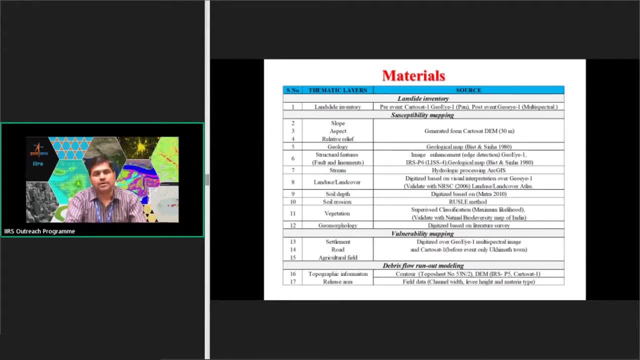 This is how I get the sustainability map. I have separately got the vulnerability map. So vulnerability map, sustainability map, if I cross it, if I cross both these, then I get what is called risk. So the risk map is finally going to get me information. 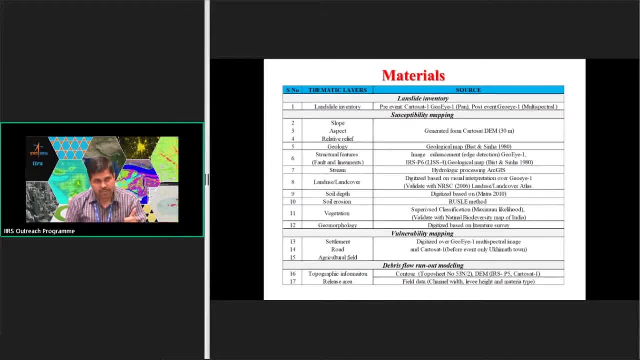 So the risk map is finally going to get me information. So the risk map is finally going to get me information about two things: Valor elements are present or not, And how much. what about the sustainability of that area? Last phase of the slides, I will discuss more about the debris flow modeling that is directly for mitigation. 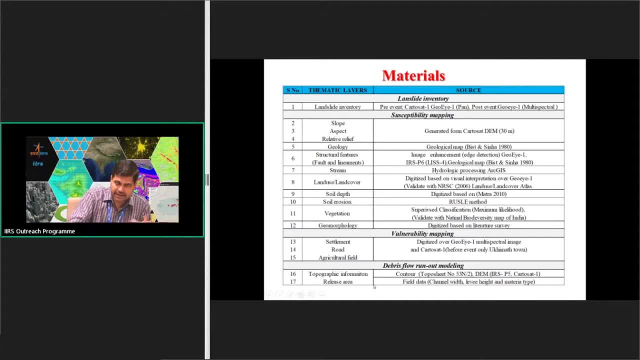 For that we have. we need the topographic information, like a DEM suppose to build, And that DEM digital elevation model. we have to know where from the landslides are happening. If I know that you know these are the source areas where from landslides are initiating, then how much they are going to flow down? 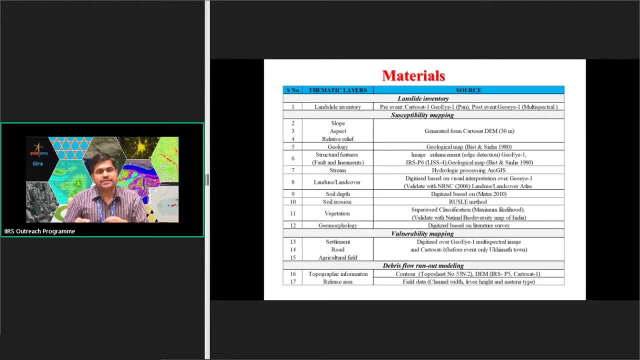 So what is the total run out? And anywhere in this spot in the run out, if I, you know, stick to a point at that particular point, what are the variation of physical parameters I can, you know, get information about from this model? four physical parameters: velocity, height, momentum and depth. 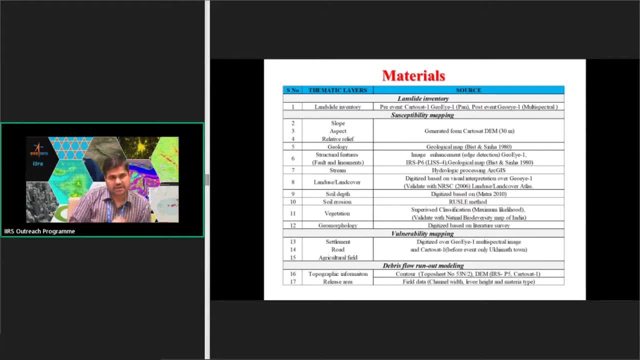 Velocity will tell me. Velocity will tell me With what velocity the material is coming down, the height, with what height the material is coming down and the momentum m into v and the pressure Pressure basically will change with depth or, suppose your, the height. 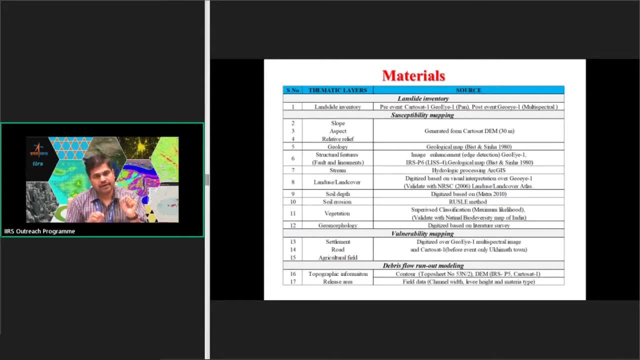 So at one point, at one xy, I can let you know that what is the variation of these four parameters and a total run out path? So this basically tells me Velocity is considered in a more flow modeling. We'll come later on to that. 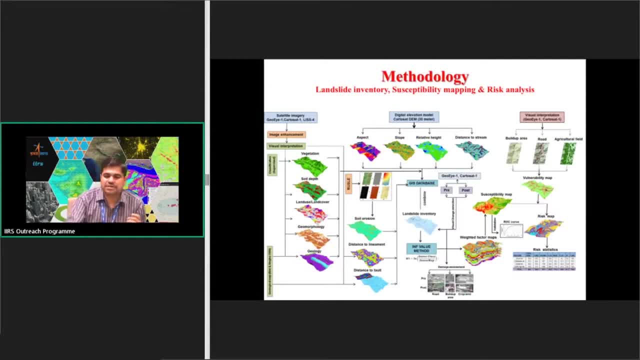 So as I was discussing the inventory one- sustainability and risk analysis- there we go the pictorial way. So different kind of satellite imagery and other sources gets me different types of thematic layers And these thematic layers, if I cross it with inventory, gets me. 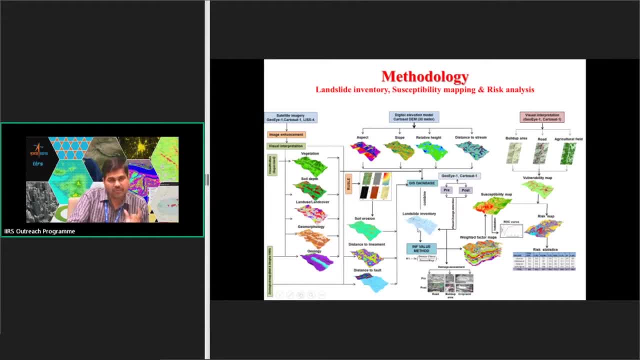 My, If I cross it with inventory gets me a combined map. If I stitch these combined maps together, I get the sustainability map. Now, sustainability map: here I get from satellite image only build up area, road, agriculture, all elements. 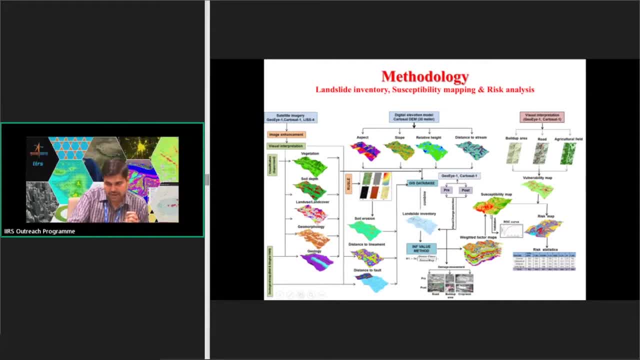 So if I combine these two, I get vulnerability map. If I cross vulnerability and sustainability together, I get a risk map. This is what I was telling before coming to the final sustainability map. The combined maps are basically weighted factor maps. They are factor maps. 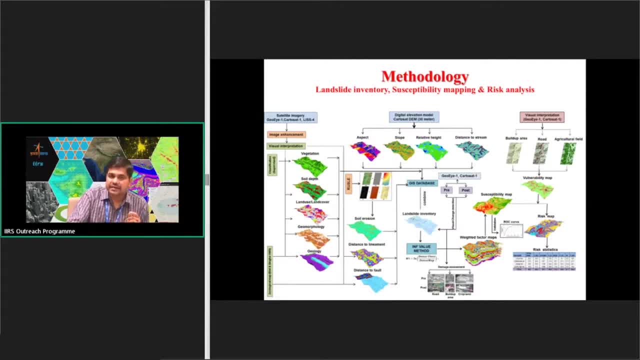 So they, each of these layer is basically: it contains information about one of the thematic layer and inventory, So so I get different factor maps. I can further give them weights also If I think that you know, suppose geology is more important or drainage is more important, like that. 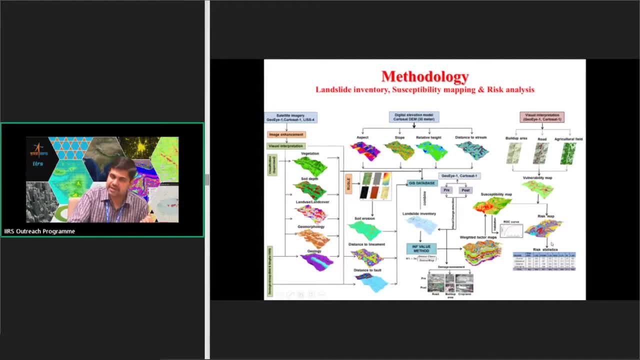 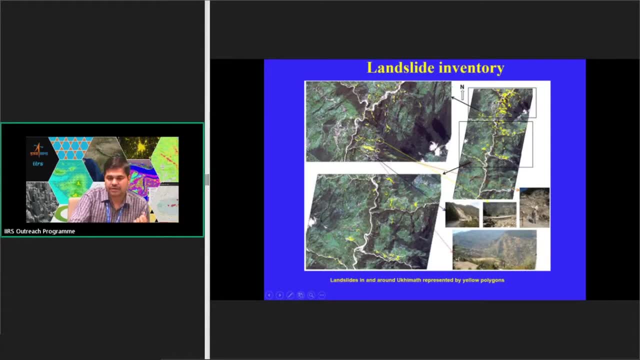 So once I get sustainability map out of this, I cross it with. so vulnerability gets me risk map. So this is where. This is how the landslide inventory making will look like. So these are yellow polygons- basically tell us where the landslide has taken place. 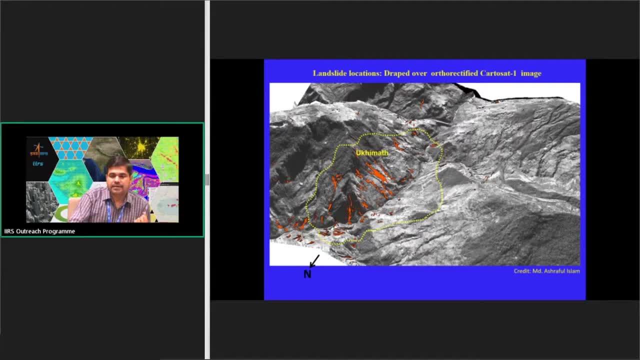 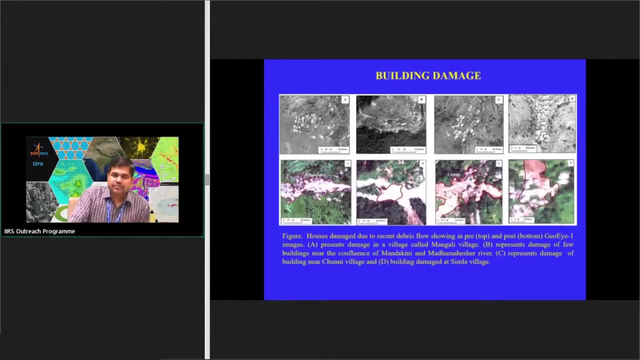 So in a 3D draping simple Cartosat 1 image, we have draped the landslide polygons onto this and see that how they are following. Next step for vulnerability calculation I have to go for building damage assessment. Suppose building is an element. 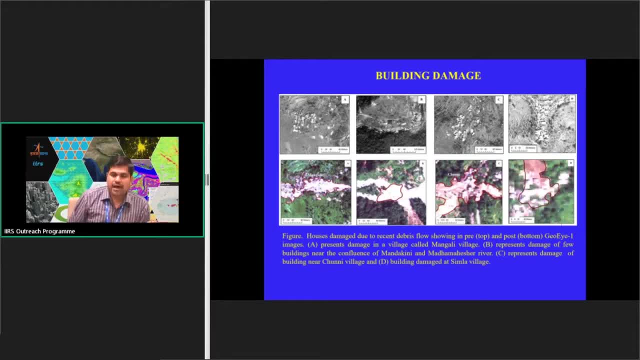 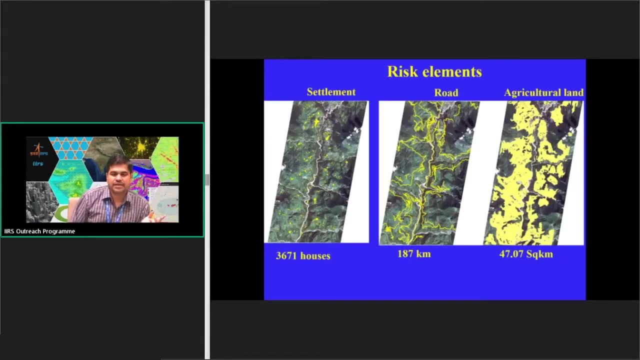 So for that building I have to map buildings, I have to map roads and I have to map agricultural field. These three if I'm taking for as elements. So if I put this together I get a. if I put the settlement, these are the settlements or roads or raster layers, and then the agriculture land. 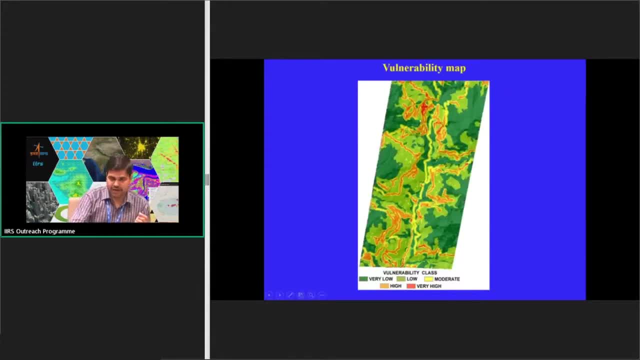 So if I put this together, give them further weights, I get a vulnerability map like this. So obviously it indicates the red zones are basically very high. So this is a classified map. Very low to very low. So this is a classified map. Very low to very low. 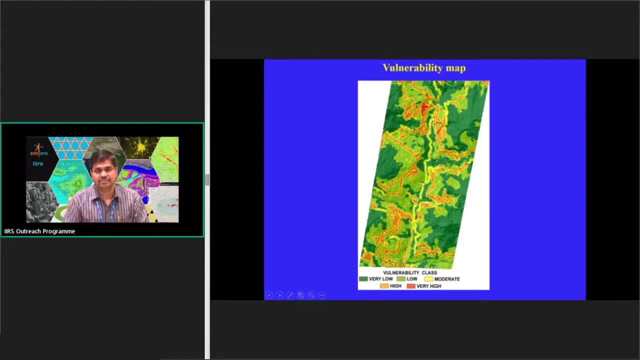 So very high obviously indicates that it has maximum vulnerable elements present contained in it. So it's quite apparent that from this looking at this only, I can tell that my roads were given maximum weightage because all my roads, all along my roads, come in my red color. 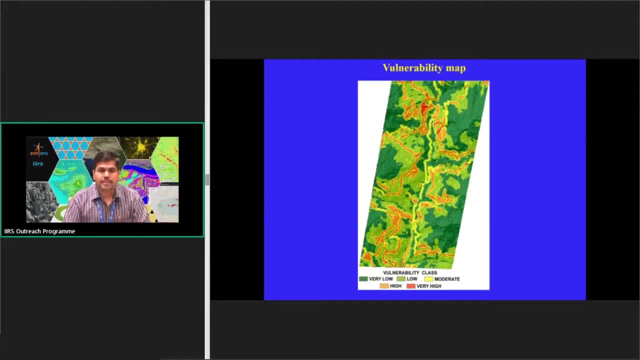 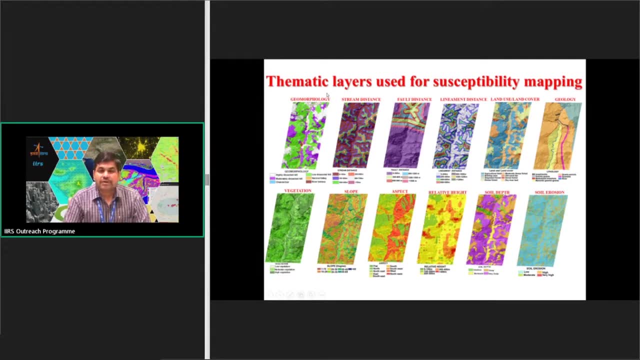 So that indicates that roads- I have deliberately put road with maximum weightage for vulnerability calculation. This is what I was telling for thematic layers for sustainability calculation. This is what I was telling for thematic layers for sustainability calculation: G-morphology stream, distance, fault, etc. etc. 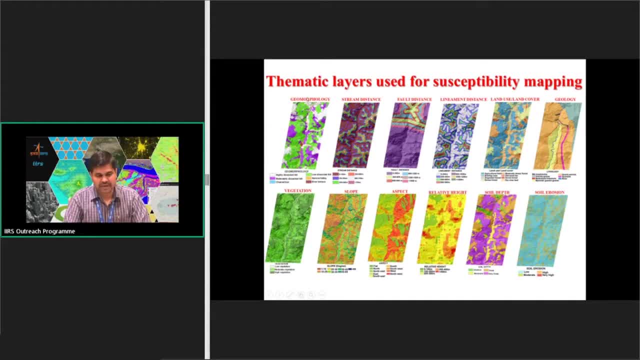 So all these supposed to have layers, Each of them will be called a thematic layer. In this thematic layer there are supposed 5-6 classes in each of them, as you can see very clearly. So basically, you have to, we have to cross this thematic layer with the inventory map. 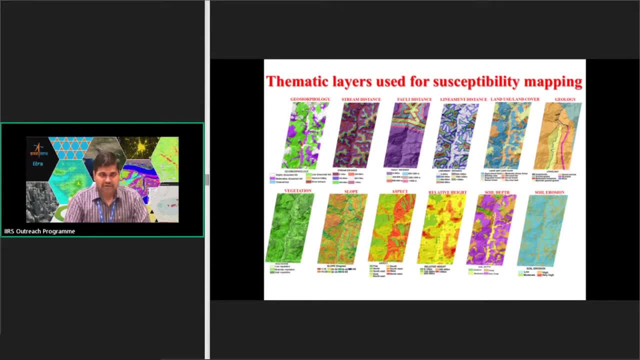 Inventory map shows you the landslide polygons, the actual landslide happening. So if I cross the landslide with this, then it tells me simply that which of these classes contain maximum polygons. so the maximum polygons contained in the class is obviously maximum influential. that is what we assume. so if it is maximum influential, 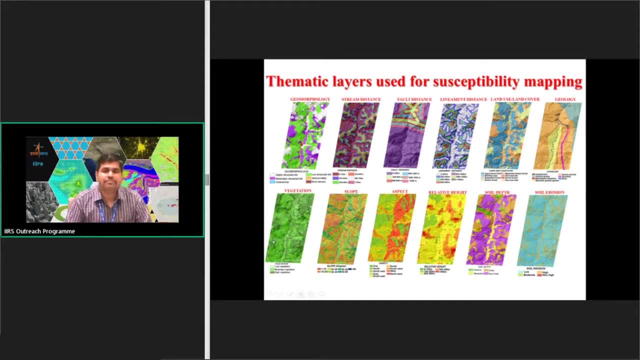 then, which will be the least influential? so, among these 12 thematic layers, i will finally come up with, suppose five, six most influential classes. one class in suppose slope 45 to 60 degree class contains maximum landslide occurrence. one class in suppose soil depth one particular type. 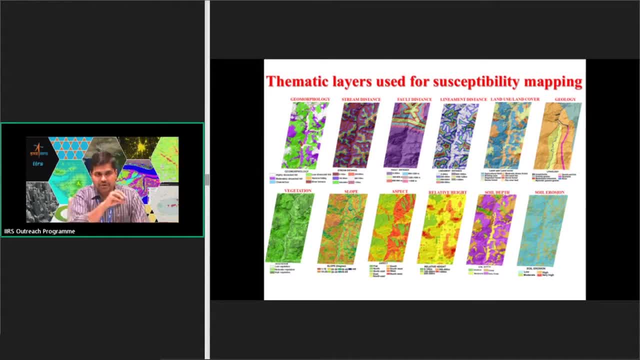 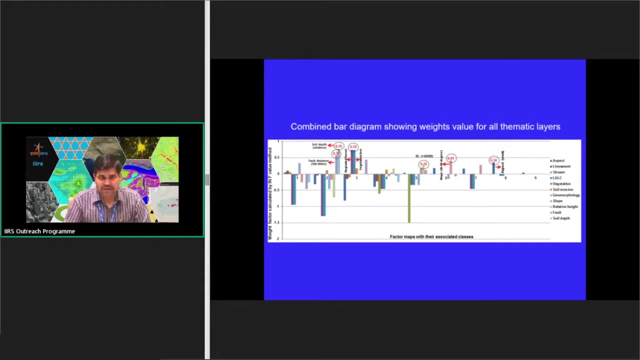 of soil class contain maximum polygons. so these one one suppose- classes, they are basically the most influential factors diametrically. if i want to show this, it will look like this: there are several ways of calculation of stability when- no, when- you approach to stitch the weighted factor maps. there are some computer generated programs, there are simply some mathematical. 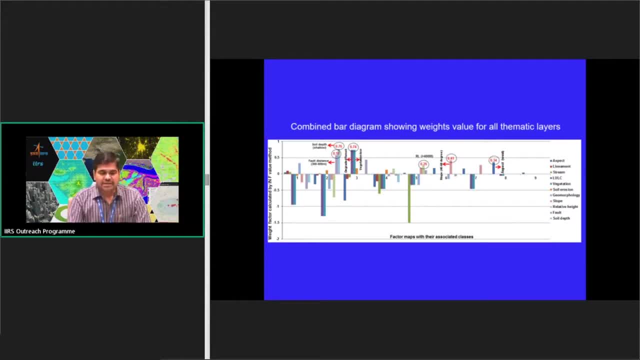 means, statistical means. there are some knowledge based means. information value is one of such statistical method. mathematical method, where information value is a factor, is a numerical that is calculated from each of these factor maps. so that tells me, suppose we have slope. slope has four classes now. the each of this class will have one one information value. 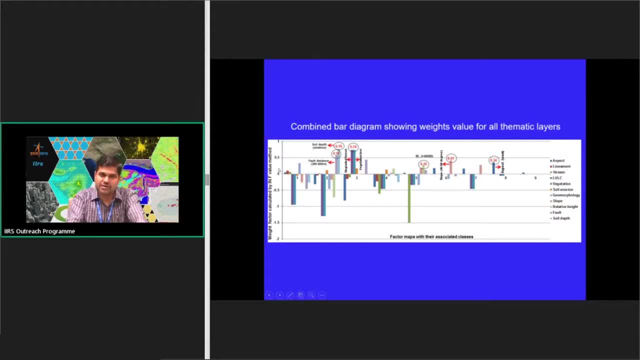 some information value will be more than zero, as you can see here. some will be less obviously. less information value that means it contains less number of landslide polygons. that means that they are less influential. so if a class contains more number of polygons, that means they that class is. 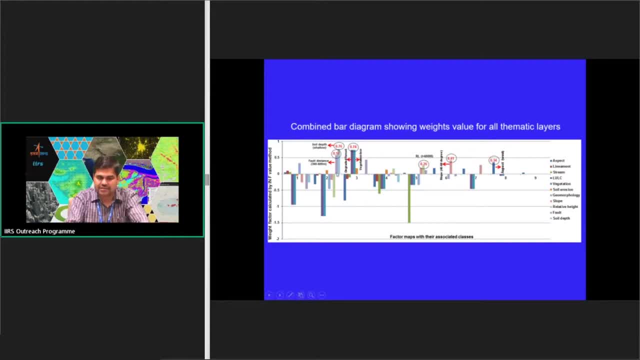 particularly responsible for, you know, occurrence of landslides. so that is given by, that is here, is predicted by a, your a high value, high positive value. so i have no. yes, there are other class class marked the maximum influential OSD values Now one, two, three, four, five, six, six. 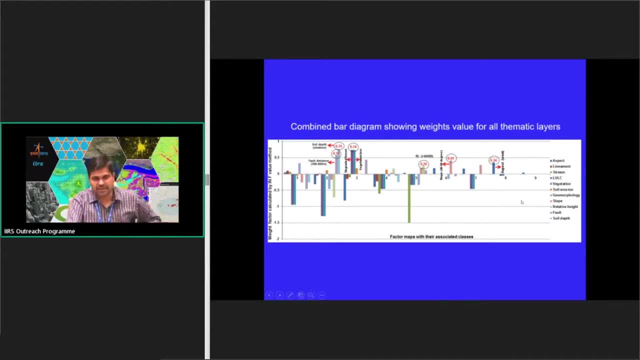 total factors are coming out from this pictorial representation which are the most important, most influential factor for all kinds of landslides in that particular area. So you can take it apart. they are the more important from the other. These are the susceptibility. 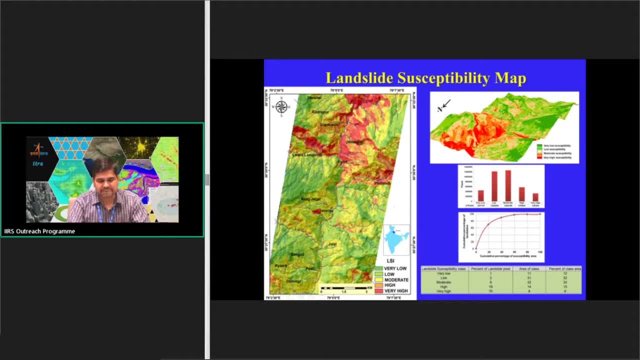 map will look like. So the map basically is repainted by again five glasses, very high to very low glasses, red to green, and you see these are the area, Ukkimat. it's very close to Kedarnath town and we have seen earlier the 3D Daping one where the maximum landslides 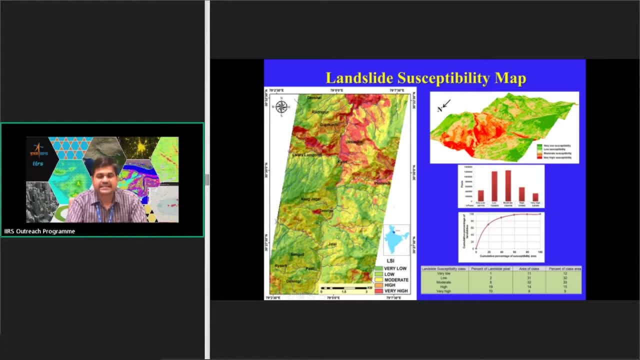 were occurring. So I see that you know, the red patches are concentrated in this area only, not here. So if it is concentrated in this area, that means that they are more susceptible. Yes, Most susceptible areas. so obviously, for validation, if I go to go to field with this map, I 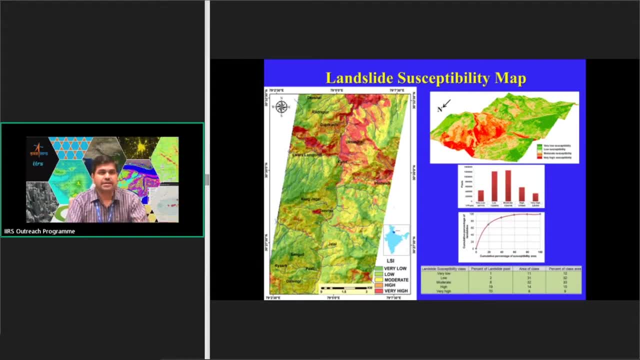 should get concentration of landslides. I should see landslides in field concentrated in these areas only, not here. If I am getting landslides mostly in this, not in this, that indicates that somewhere somehow I have committed a mistake. Can be a calculation mistake, So it can be the classes. 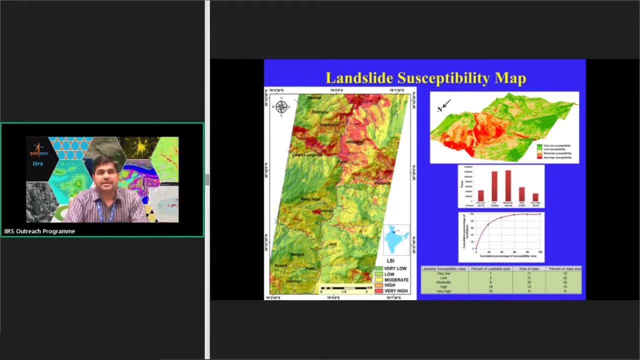 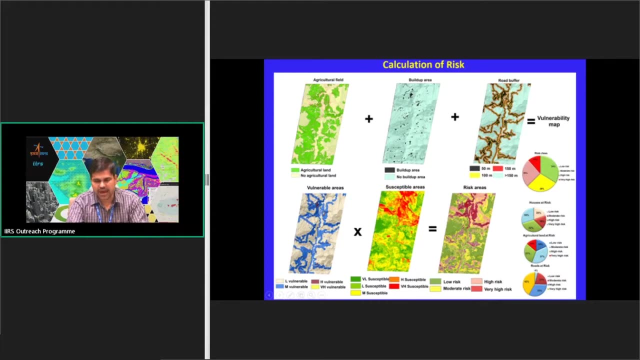 The thematic layers that I have taken were not appropriate. Maybe that I have taken more classes or maybe something important I have missed. So all these I have to examine one by one. So this is how, in totality. So there is a vulnerability map and agriculture built up and road buffer. 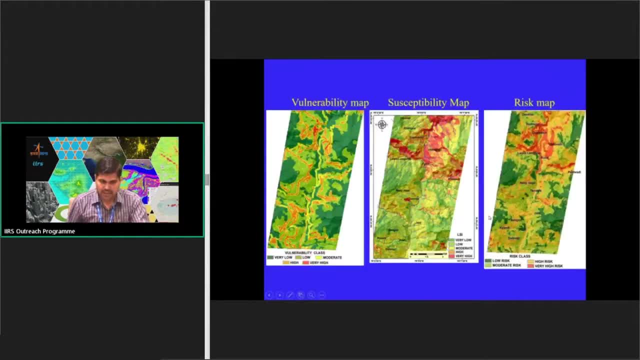 Then vulnerability area into susceptibility gets me risk. So side by side I have to check like this: I can get off one, I can stick to one area. This, X, Y, I should check the susceptibility, I should check the vulnerability. 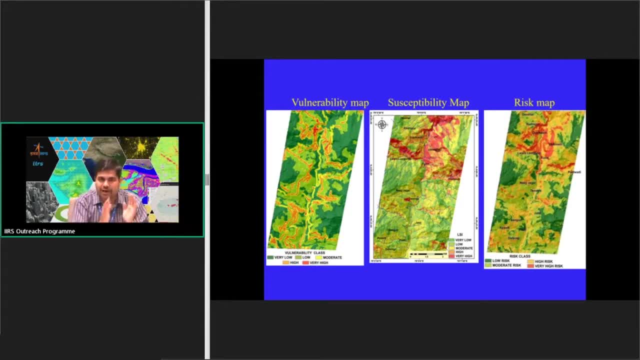 Just to get an idea which one is contributing, which one of the vulnerability and susceptibility contributing more to increase in risk? enhancement of risk. So risk is getting enhanced because of vulnerability or susceptibility or both. So it is a pictorial idea that we can get from it. 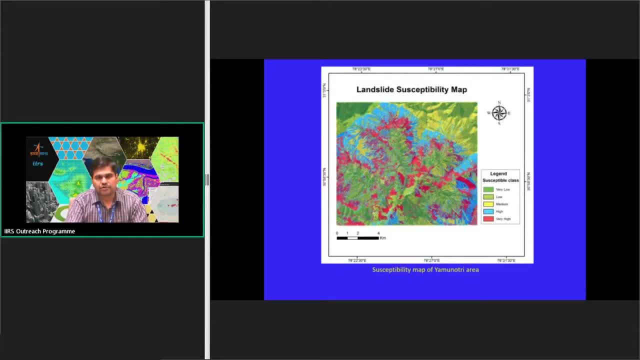 Similar studies we have conducted by our students Here in IRS different study areas. Some of the slides that I presented were done by the past students of these institutes only, And this is one of them. suppose This is from Yumunathri area. 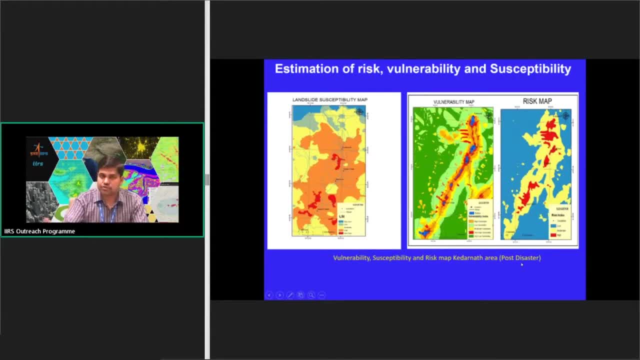 This is from Kedarnath area, but it is post-disaster, That means post-2013.. So we tried to make an attempt that how does it look different from what happened earlier, Early 2000,? we had a map that I started with. 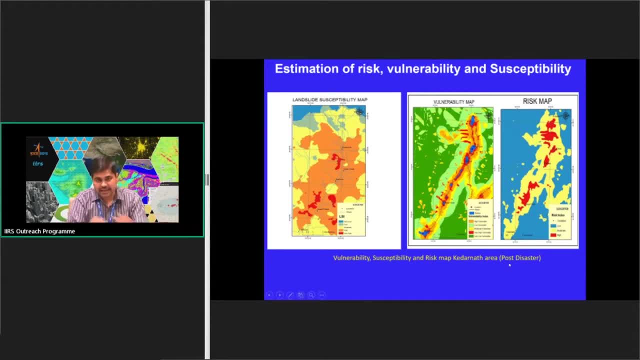 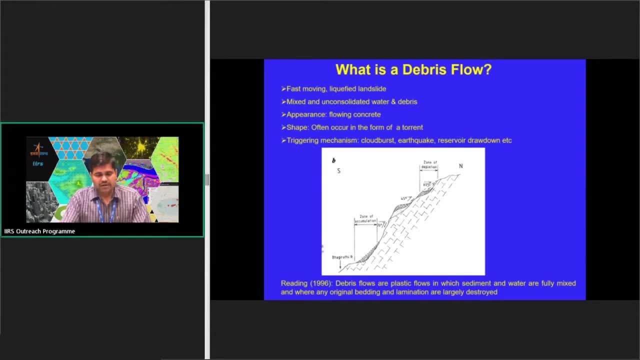 And now we have. We have another set of map. So that is post-disaster, So any change is happening in susceptible, vulnerable classes or it is the same, basically, Further proceeding into my today's lecture, So I told that once we are done with the risk parameters, we have understood the risk parameters. 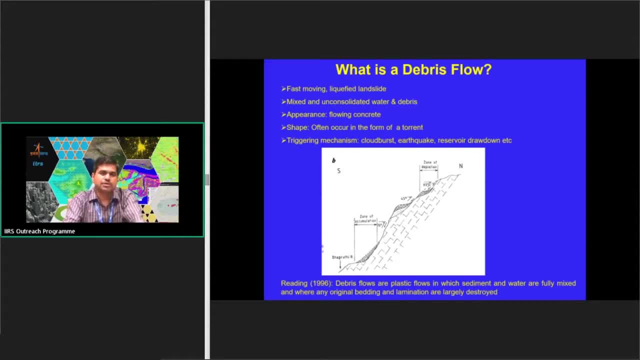 We have known how to assess it, how to monitor it. Now on to the mitigation part. How do I mitigate it? So what is about the mitigation? Suppose I have come up with a sensitivity map or a very good hazard map. I mean vulnerability map, suppose, or a risk map as such. 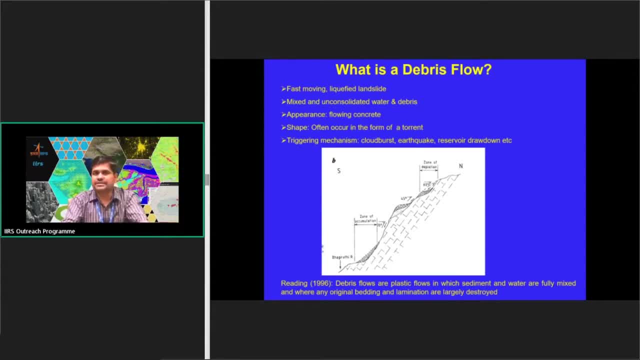 So if I have that in my pocket and I go to a village, in a poor, I mean in a remote village where it is cut off from rest of the society, suppose, but the area is very much prone to landslide. So I know that though this area is 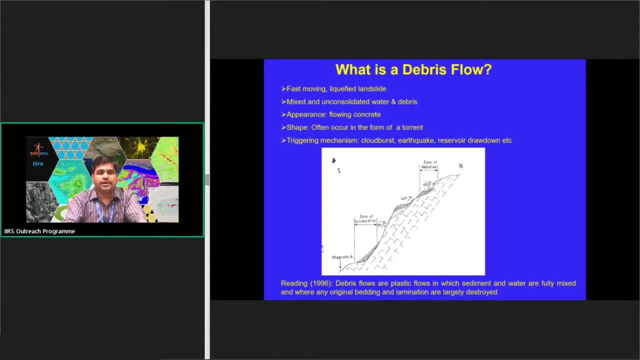 So I know that, though this area is prone to landslide, So I know that, though this area is falling under very high risk zone, what do I do with that? What is my next step? Can I do anything with that? So, for real mitigation if a landslide happens, only knowing that is not going to be sufficient. 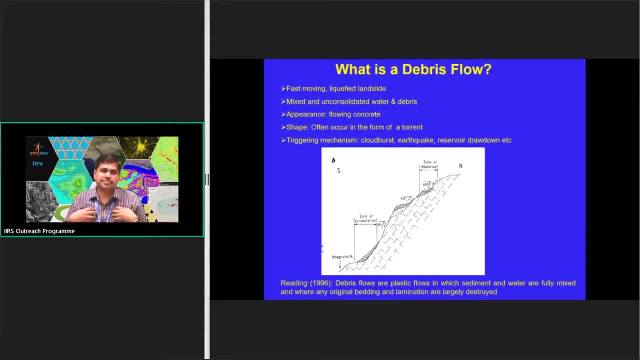 If I know I have a disease, if I know I have this kind of disease, is that going to help me? No, I have to get medicines to eradicate that. So the modelling kind of things. They are basically loyal, Okay. 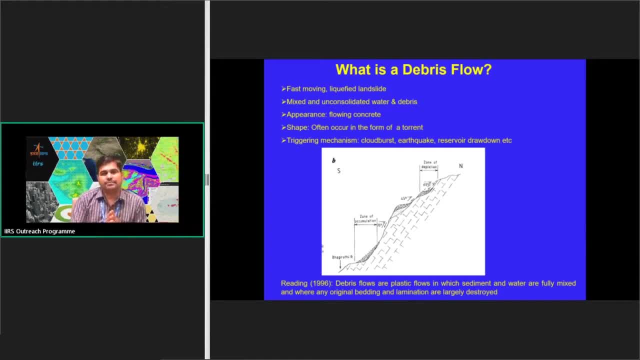 medicines for this. so this will give you and predictive, futuristic approach to know beforehand that this can happen. if I know it beforehand, then this can happen and with this much of extent I can definitely prepare for you know some remedies, so what they are, we have, we're taking into consideration here a flow. 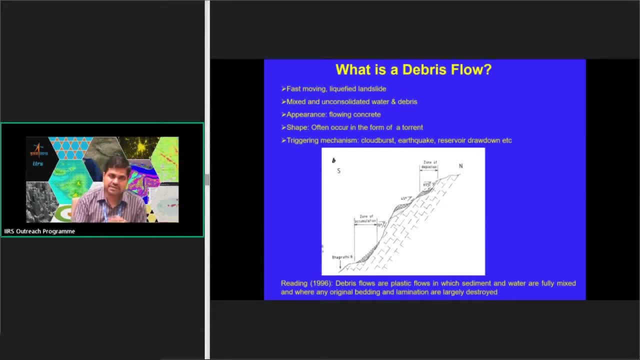 only as such. you know. I have described what the flow is. it's mostly your debris material will be involved. so debris is a rock chunk embedded in clay matrix and then full of water. so they are fast moving. very liquefied flow because of water. they are mixed: unconstituted water and debris. the shape is often like a 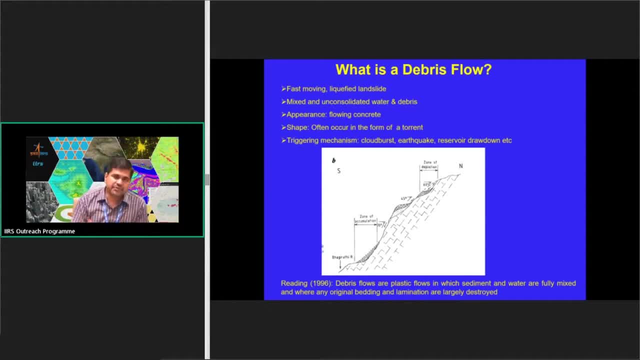 torrent or a drain kind of thing, and then they can be triggered by a cloud burst, sudden rainfall, suppose an earthquake, seismic movement or a reservoir drawdown. so all these taken together, I understand what a debris flow is so in a cross-section, if I want to understand, so this will be your. 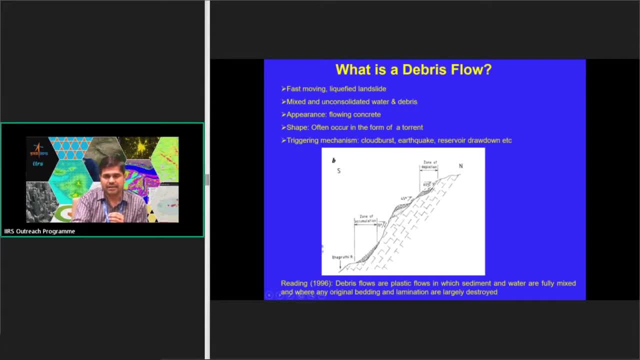 your flow. if you want to understand, so this will be your flow. if you want to, where from the material is coming, so this is your zone of depletion and this is where you know the material is dragged down and this is where it gets deposed. suppose the river is somewhere here. 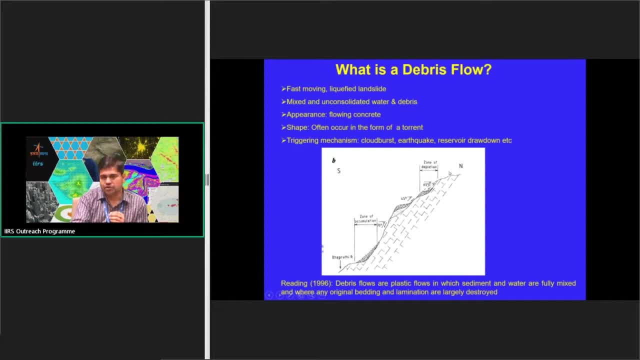 so zone of accumulation, zone of dragging and then zone of your source. yeah, so in. in short, it will look like this reading: as such, in 1996 defined every flow are plastic flows in which sediment and water are fully mixed and when they when where an original bedding, original lamination. 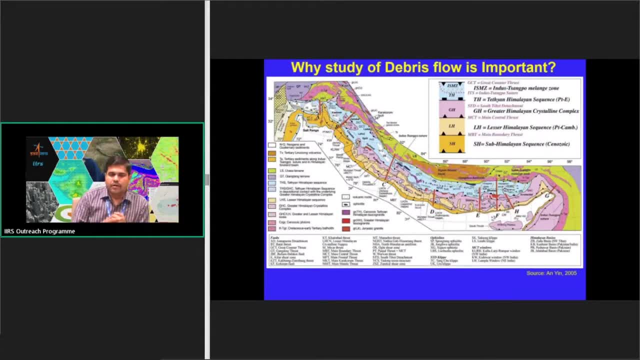 is largely destroyed. you cannot get it back. why do i study the debris flow? why? why it is important because we have to understand. suppose this lecture is being delivered from uh. there are the units, it's the lap of himalaya and then in between, sandwiched between your uh, shivali kimala and lesser himalaya. 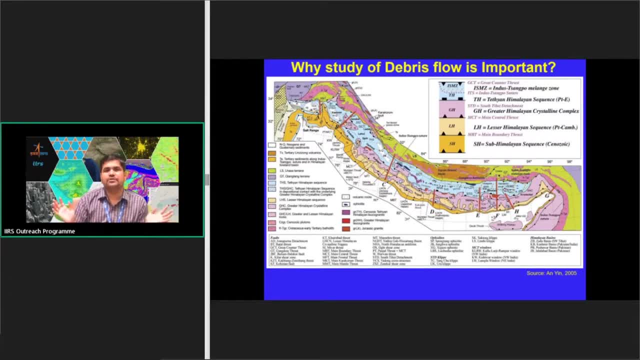 so there are chance, chances that you know, anytime you know, large earthquake may hit this area. so with this potential seismic hazard, uh, there are triggering mechanisms already ready. so if my triggering mechanism mechanisms are there and the already landslide prone areas may get again activated very soon because of this. so that is how? uh, the study of debris flow. 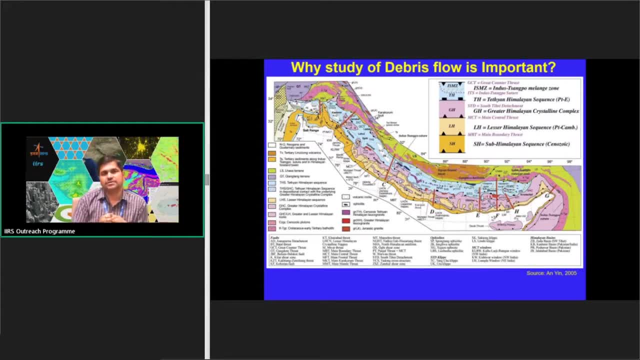 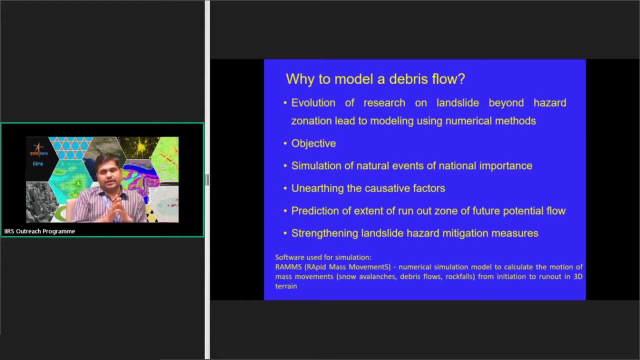 is important in terms of rainfall. also, this area, you know, receives severe rainfall in monsoon and the seismic factor. so taking these together, uh, makes my study of debris flow important. now, how do i model a flow? what are the criteria? uh, i'm sorry. before that, we need to understand. 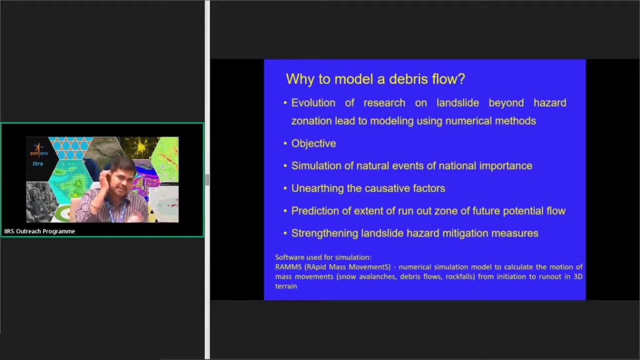 why do i model the flow? what is the need of that? so, evolution of the research. we have seen that landslide has reached beyond hazard generation and now we are on to the realm of mitigations. so it's mainly objective. the why the term objective is coming, because landslide hazard. 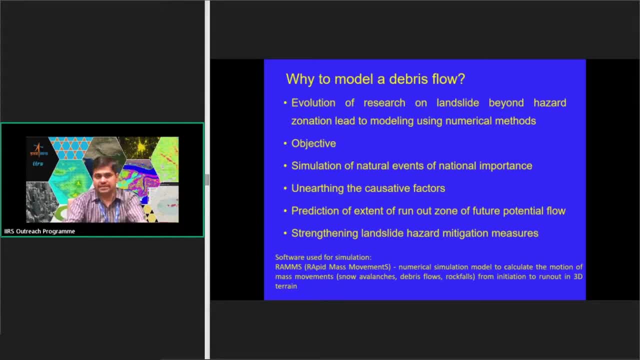 generation map preparation had a lot of subjectivity in it, inherent subjectivity in it. what do i mean by that? because somebody is doing a map, preparing map here and somebody in some other continent for the same area using same satellite data or some other satellite data using same mathematical calculations or some. 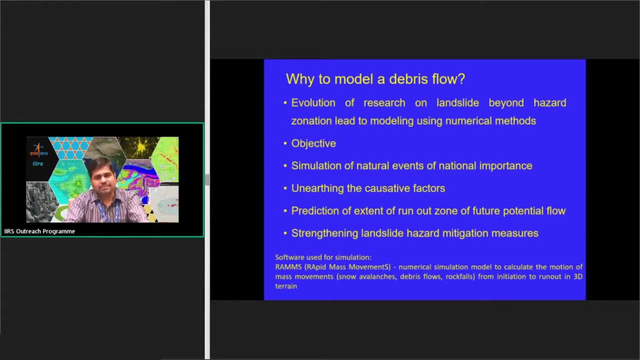 other is going to give me, at maximum places, slightly different results. so why this difference? why this subjectivity is creeping in? maybe because of the mathematics is not allowing the result to be same or the data input is not same. so that is why the subjectivity is there. 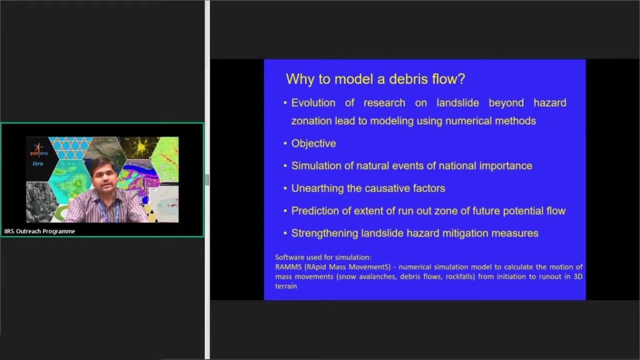 but how to get rid of this? if we model a thing, it has to be objective, because it's completely mathematics based model, physics based model, and it doesn't vary spatially or temporarily. so what i do here today- and somebody does it, you know, sitting a thousand kilometers apart- 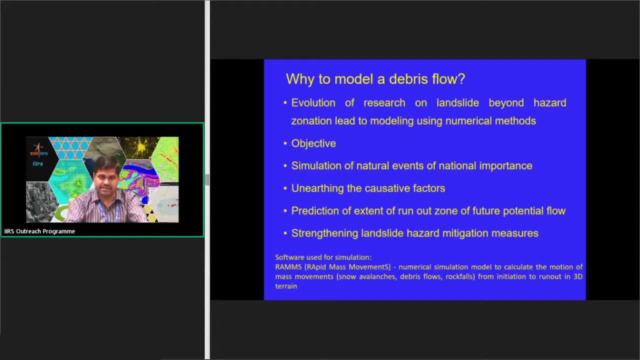 from this place is supposed to, we're supposed to get the same result. that is why it is objective. then simulation of natural events of national importance. there are many national, nationally landslides which has to be simulated, modeled in laboratory. then it another cause, the causative. 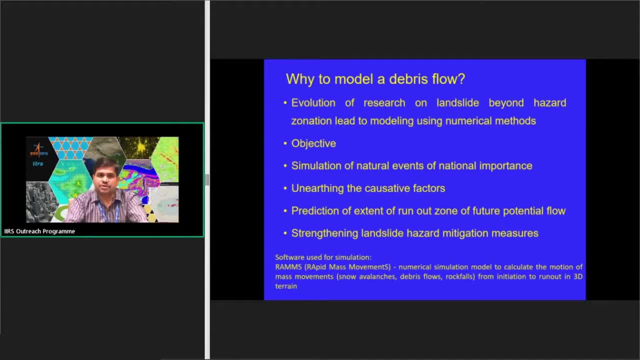 factor. so we very closely, we can see which are the factors because of what the landslide was happening, then the prediction of extent of run out, as i have told earlier, and there is a future potential flow. so future, in future, if that landslides gets reactivated, what will be the flow? 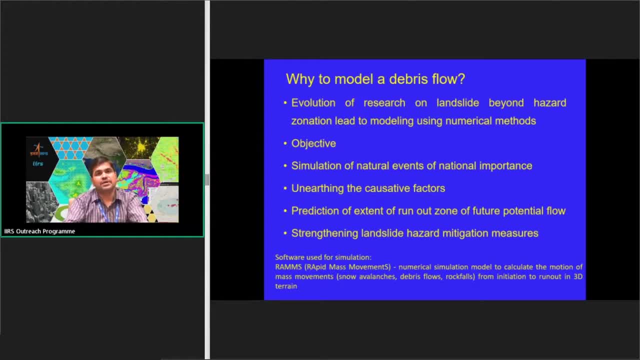 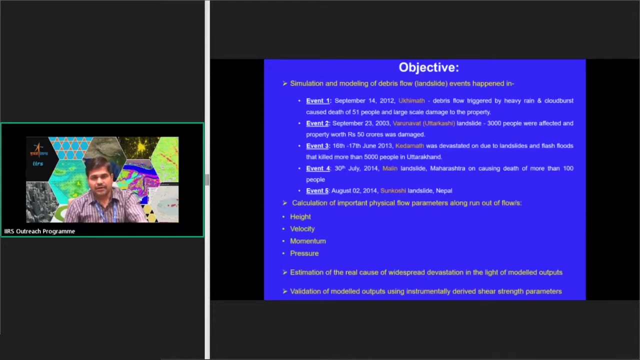 up to how much distance it's going to cover. what are the villages that will come up in its- you know- torrent and may get, may potentially get, destroyed and then thereby strengthening the hazard mitigation measures. we here, we use a model called rams and we have using this, we have modeled many 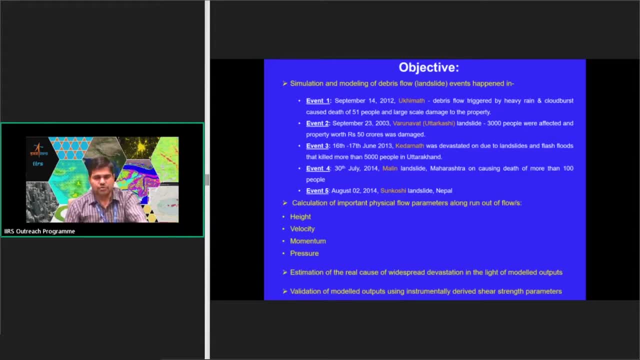 events. we have listed here only five of them. so ukima 10- 2012 event and there are around 50 casualties. then event two: barnabas in utarkasi- landslide. so though the casualty was not there, but heavy loss of damage was there. then kedarnath event 16- 17 june 2013. it created a havoc in this state. 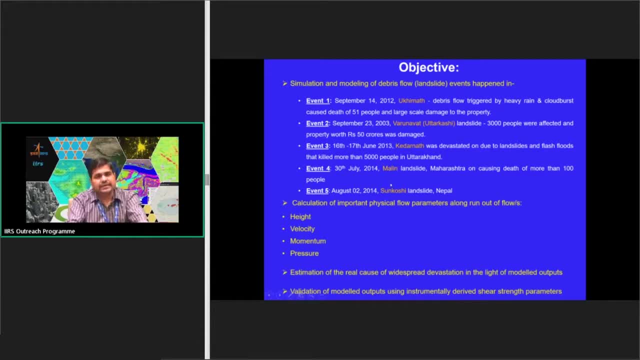 then we took a malin landslide in, you know, in sankoshi river in nepal. then we have taken in, taken some one, sorry, sorry, malin landslide is from from maharashtra, in india only, and we wanted to basically see that you know how the material, how the rock type are different from himalayan region and the basalt, so sahadri. 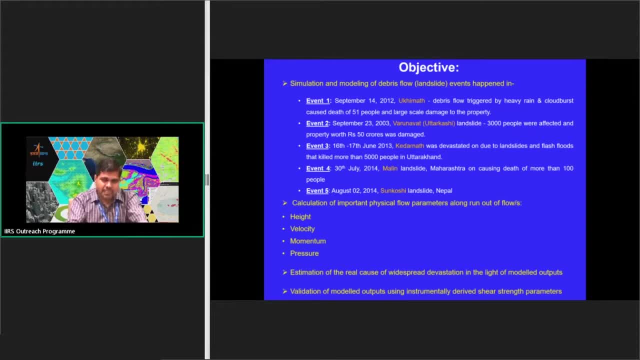 hills. basically, they're mainly decan basalt. what is the major causes of landslide there? if i, you know, apply the same model in a basaltic region, whether it's going to give me the same similar type of results, successful results like what we got in himalaya. 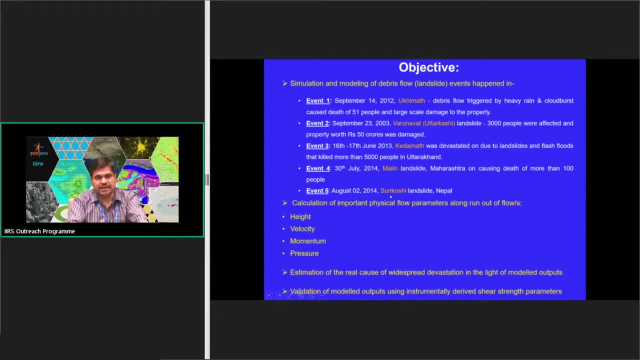 and then the sankoshi landslide in nepal. so it's basically uh, the sankoshi in due turn becomes a kosi river in bahar. so whatever happens in sankoshi, we have a effect in bihar partial. so that is why we were required to study this. most of the works are: 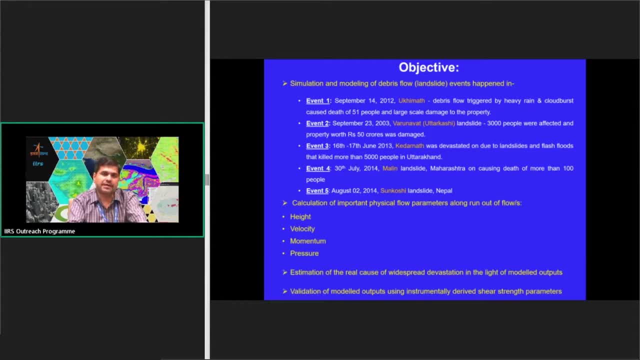 published in literature. so if people are interested they can mail me and get the papers also now, as i've told earlier, there are physical flow parameters that are very important and all along the torrent, at any point, we can get to know about them. what are they? they? 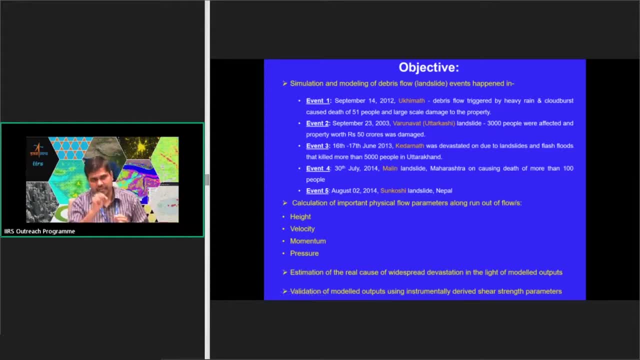 are basically the height, the height of the flow it's coming with at any point, and the velocity. with what velocity is coming in? centimeter per second, suppose the momentum in meant to be. and then the pressure, what pressure in kpa, kilo pascal is coming, coming down, and then evolution of the 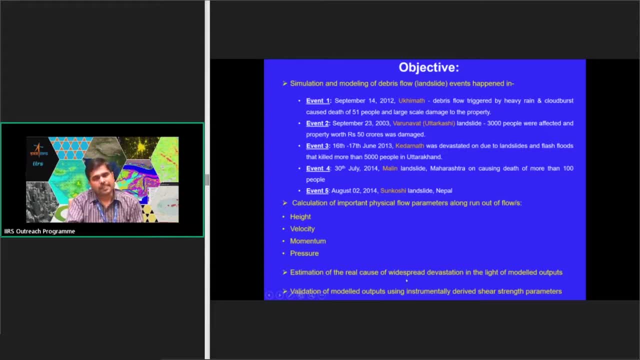 real cause of widespread demonstration, etc. we can get to know. finally, we can validate the result. we have got a very good result, but how do i know they are correct? so we go to field uh assuming uh the same uh saturation label. we collect samples and then, and then um in the lab, we analyze their. 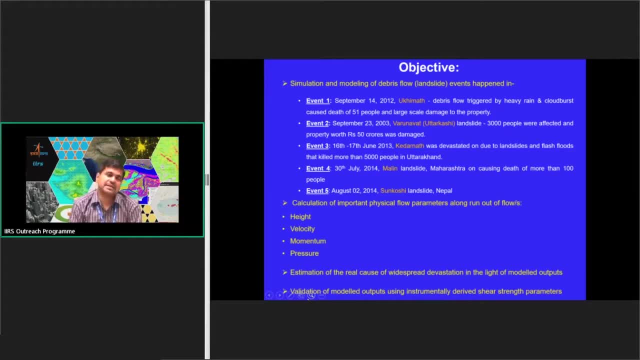 strength parameters just to see that whether the strength parameters derived from the raw, that we correct from the field, are similar to what we give as input to the model. so for running a model, this kind of model, we have to give several inputs. few of these inputs are geoengineering parameters, so these geoengineering 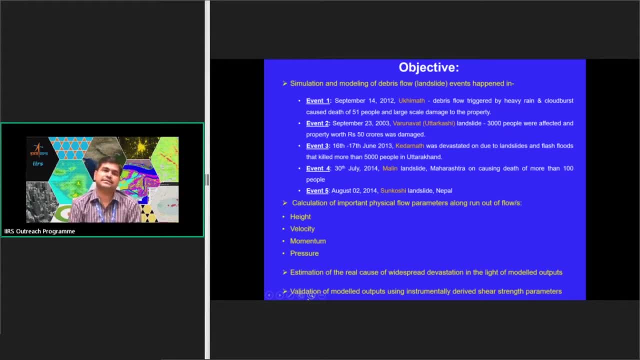 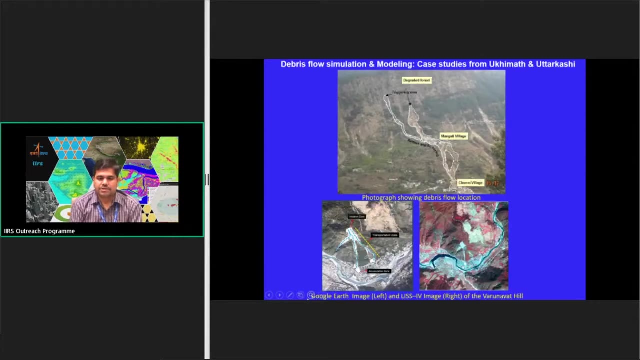 parameters are something that we can get back from the field collected samples- see field collected samples- and the input are at par, they are comparable. it tells me that, okay, the model is authentic. there are other ways also to get the check, the validity, i will discuss in detail. so 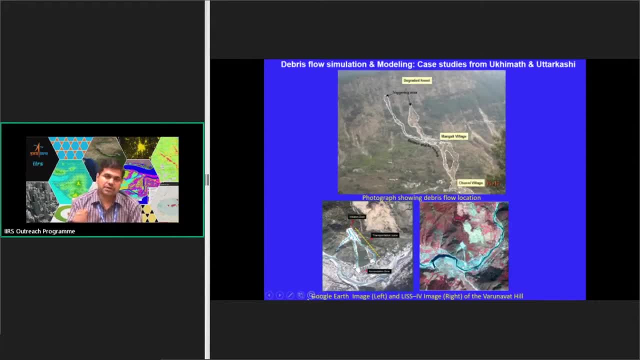 this is a landslide that we are going to. we have tried to model a nokimat town close to you can see the slide how it is. you know, this is one source area. there's another source area. there are two villages and both of them got destroyed and then it went down. there is a 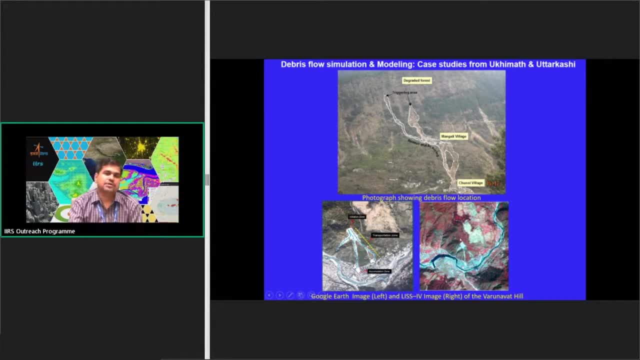 bifurcation, it went down and got deposited vanilla. this is from uttrakasi. there's a trifurcation of the landslide and you know this is how, in least for image, it will look like this and in in your google earth platform image available spotting image, basically. so that will give me a a, a better resolution, your. 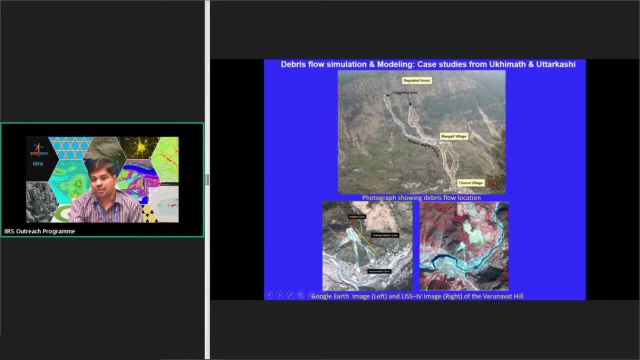 clarification. but when i do a modeling onto this, my model necessarily has to follow this type fabrication pattern and the exact extent of that. you have to run the model several, several times just to make it happen, make to make it follow the exact torrent, as it has happened. 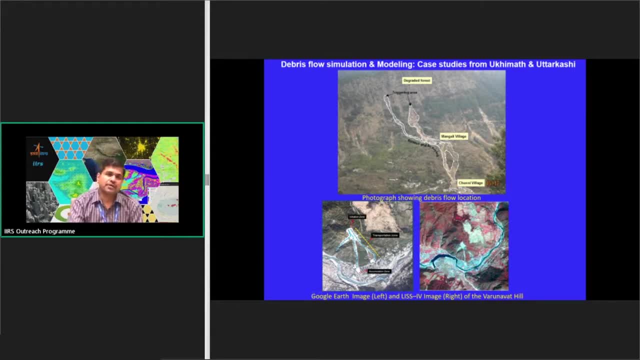 naturally so. there's one kind of validation: the moment i know that it's going somewhere else when it was where it was supposed to go. it's not going, so i have to stop then. and then i have to check for my input parameters so that they are correct or no. my dem is correct or no? 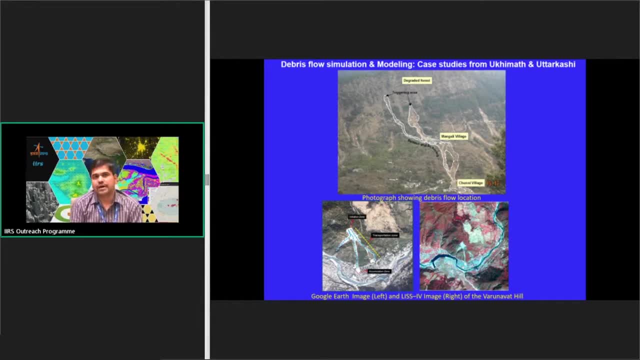 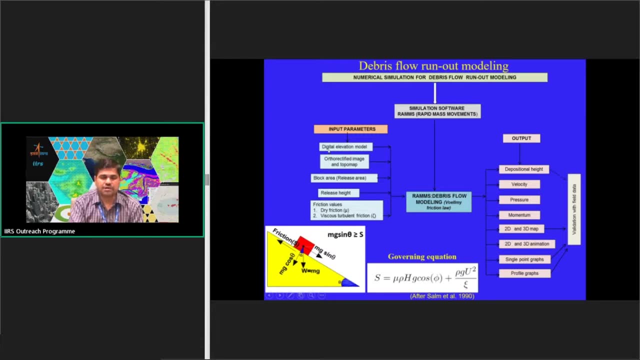 so that my exact torrent follows what happened, naturally so as for the inputs, we have discussed a lot about this. let us see what the inputs are with. the inputs are basically a dm- very good resolution dm. this particular software doesn't take anything less than, anything more than 10. 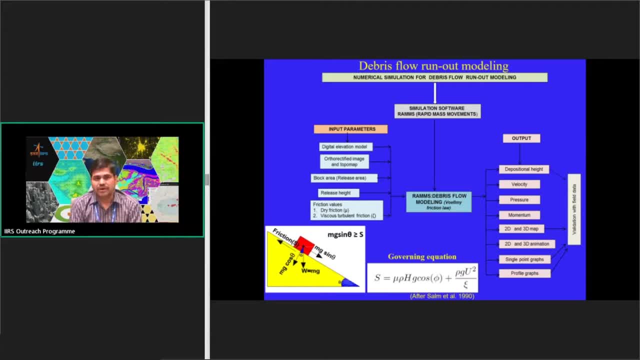 meter resolution, dm, so it has to be less than 10 meter final resolution. if it is like that, the model will take a subset area of that where the landslide is situated. and the next is you have to got some authorized images, satellite images, just to know that you know what is the source area, etc. you have 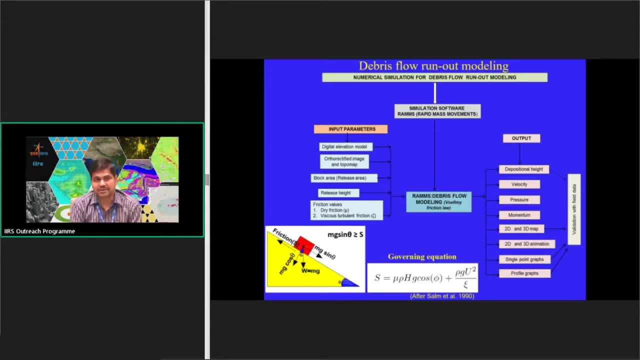 to go to the field, also before the, just to collect data. what is the depth of the landslide, where, from the source, from the landslide initiated? uh, so that is what the block area, or release area, the release area, is of utmost important because that is something that you have to physically 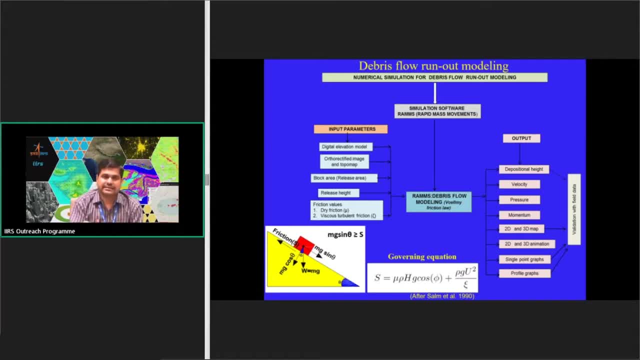 measure in the field, or you have to understand it and delineate it on your satellite image. and the same thing, same polygon, you can drag into your dem. then the release height, if the source area is quite high, suppose quite big, so there will be difference in release height. so because it is occurring on a slope and this is my source area, so 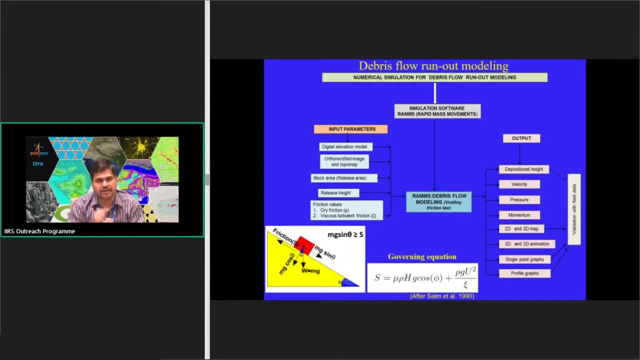 the difference will be there. so what is the average height at the release point? and then there are some changing patterns, parameters that i can check, uh using lab methods also. so they are basically two: frictional coefficient- dry friction, and turbulent, uh, viscous turbulent friction. so if i put all these as input to the software, the software. 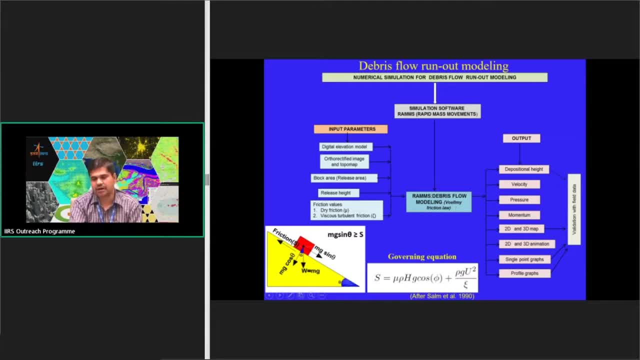 uses friction loads based on friction model only and gives these are the outputs. what are the outputs? uh, the height, the velocity, the pressure, momentum and, uh, the different type of animations, maps, etc. so what exactly happens in this? the physics of this, uh we have, has been depicted in this. 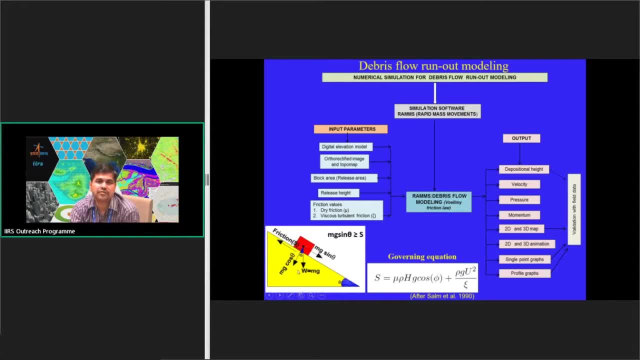 photograph. suppose the red block, basically, is going to come down and it has a weight of uh, mg, w equal to mg. so the force that is dragging it down, uh towards because of gravity, is mg sine theta. so mg sine theta is being opposed by the friction, the 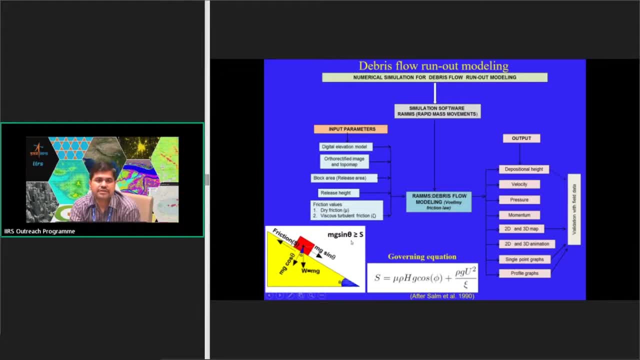 friction is represented by total friction s. so total friction s is nothing but what? what the total friction is? because this is the debris flow. there will be rocks, there will be liquid, both. so the friction because of the rock component and the liquid component will be separate. so i have to add this. so this is what the total friction is: the the total friction s. 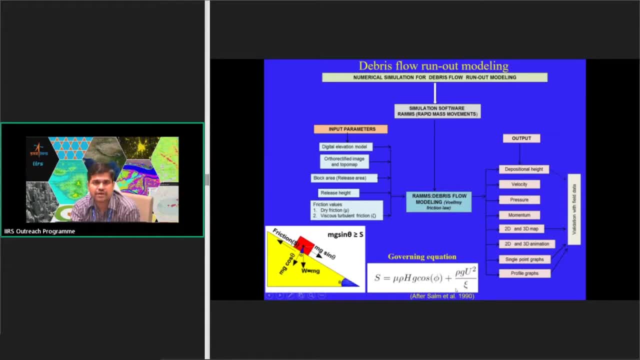 is the friction due to the solid phase and the friction due to the liquid phase. so if i add this up it gets me the total friction. once that is that we have total friction, we have calculated uh, and another software calculates that mg sine theta force. so there's a. you know the comparison. 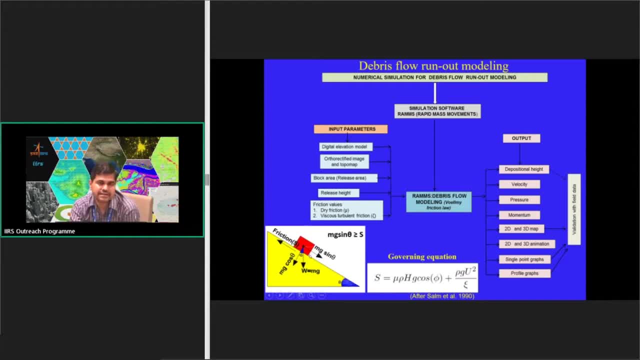 between who whichever is greater, which one is greater? if mg sine theta is greater than equal to this, then slide will happen, shear failure will happen and slide will happen. so what it exactly is the solid phase, the friction is, mu is the frictional coefficient, that is the. this is the. 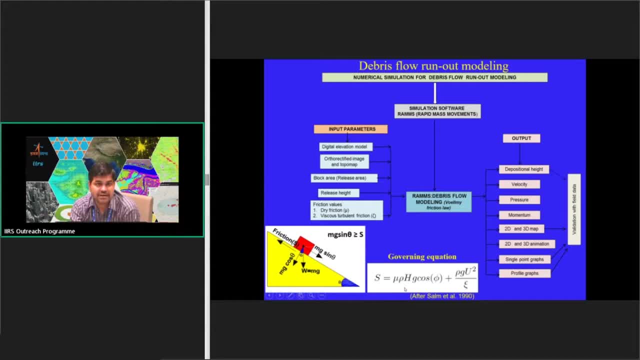 the friction. but the friction is g and g and u is the initial velocity and what that actually is when we consider it as the effect of the liquid phase that you have to give as input. uh, the rho is the density of the material, the rock, and the height is the average height. 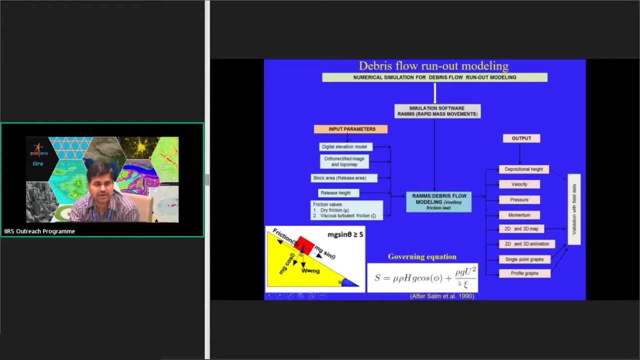 of that area, the source area, and your uh phi is nothing but theta. only is the slope. and similarly, here, rho for the liquid phase, rho is the density of the liquid water slurry, basically g, and then u is the initial velocity. initial velocity is what? if you consider of a, consider a. 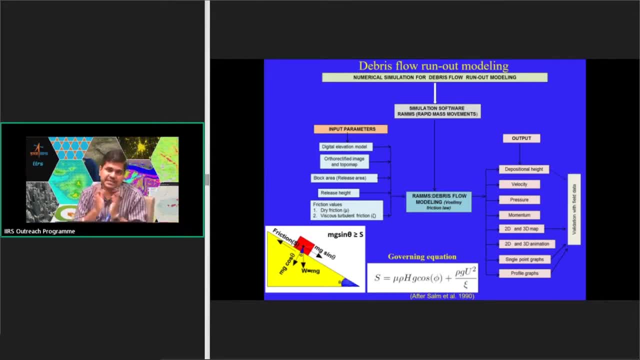 when, when this point comes to this, it will gain a velocity. so that is basically the initial velocity u it in maximum cases. we do not consider as zero as such. so and then psi is basically your dry pixel. viscous, dry, turbulent friction. so viscous turbulent friction. psi and mu, they are the 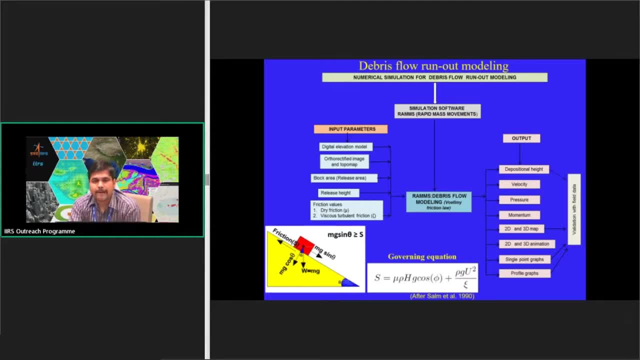 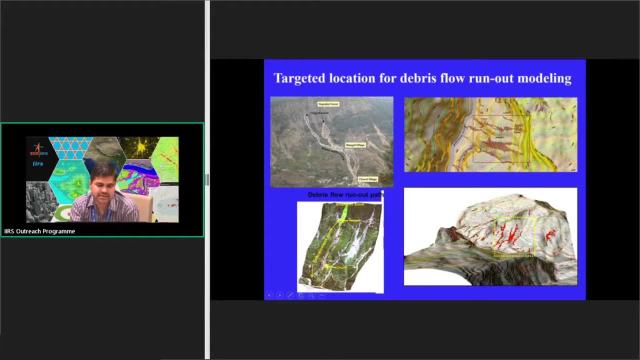 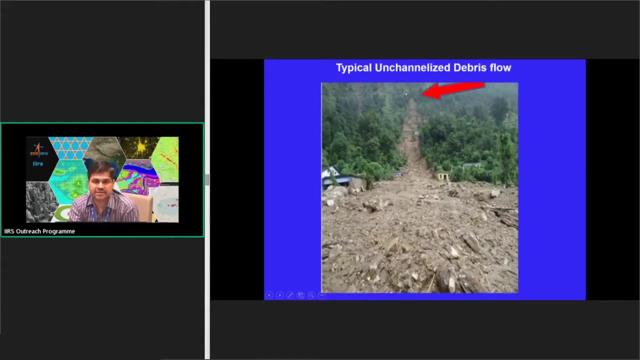 engine geological inputs that you have to give to this model just to run the model. let us see how the how it look like. this is the source area, initiation zone, and it will follow along this torrent, suppose in field. we went to field and we have seen like this is the source area. 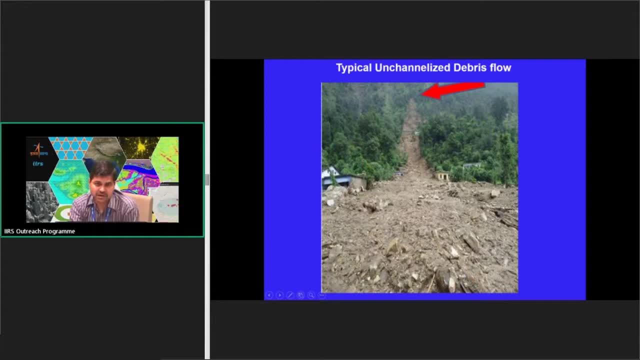 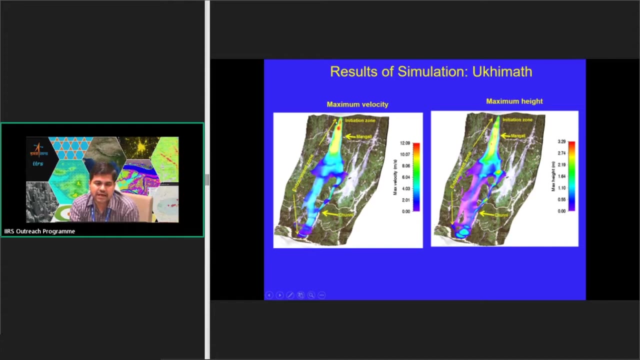 in ukima town, and this is the building that still remains. uh, all along this there had been buildings, markets, etc. so they all got devastated. the nothing remains. the modeled output of this area is like this. so this is how, uh, the velocity varies all along till it reaches the depositional area. 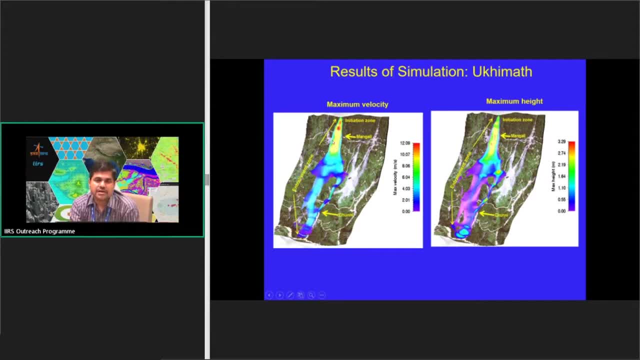 so this is one location of one village, this location of another village. now, at any point you click, you can get to know about the velocity in terms of meter per second. similarly, height: at what height you are going to, at what height the material will come down, with what height? 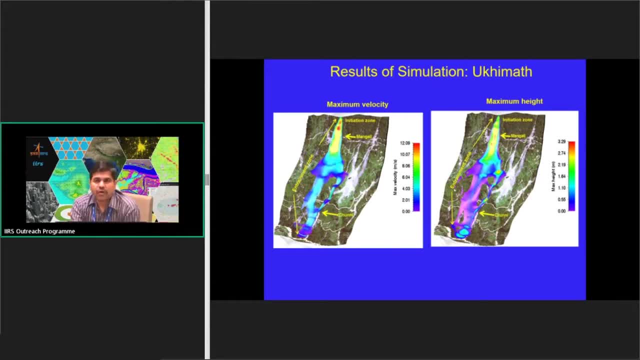 uh, how much material? uh, you can get to know. so why this is important. height information, the velocity information is really important because suppose it is crossing the one road here, this you can look at, this is a road, basically. so at the source. or suppose this road, so the material has is coming. 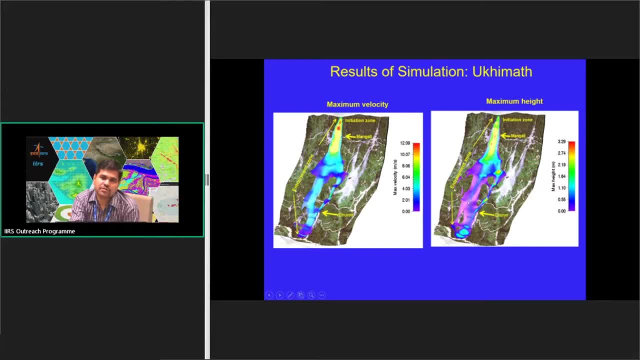 down and it, you know, struck the road with a particular type of particular height and a particular velocity. if i know the height, just before reaching, uh, the road, if i want to implant a dam, kind of thing, just to check them, kind of thing, just to, um know, check them, kind of things, so i want to tell you 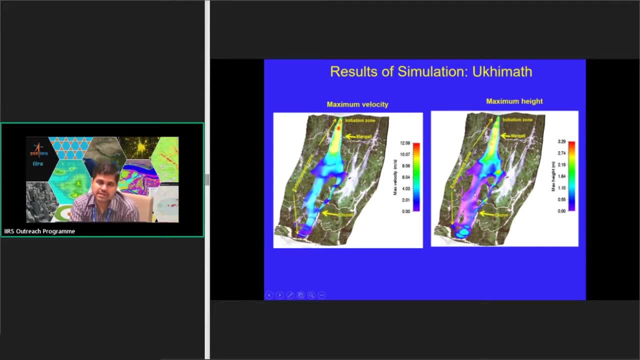 that the material that is coming down the velocity is arrested by that and that stops instantaneously there. it doesn't reach the road anymore, does it? the road before that i want to implant a dam. so what will be the height of the dam? the height of the ram should be more than the height of 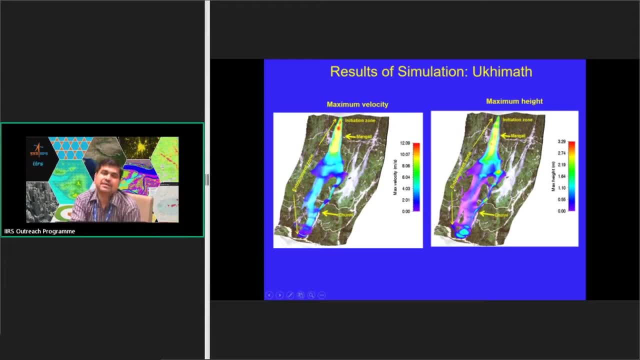 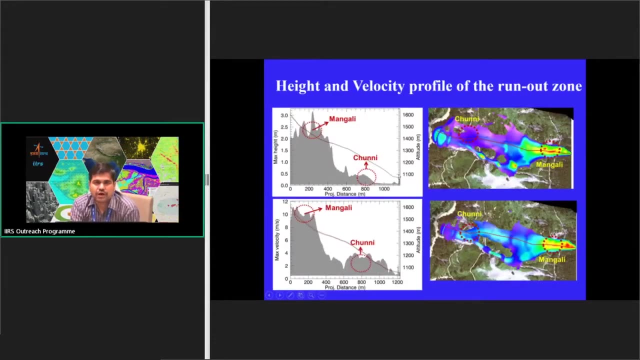 the flow. so if i click here i get a height, suppose three meter height it is coming down with. so obviously i will make a dam more than three meters so that it can sustain, otherwise that will also break and get washed away. so similarly, from the source area to down there, i can make a profile. 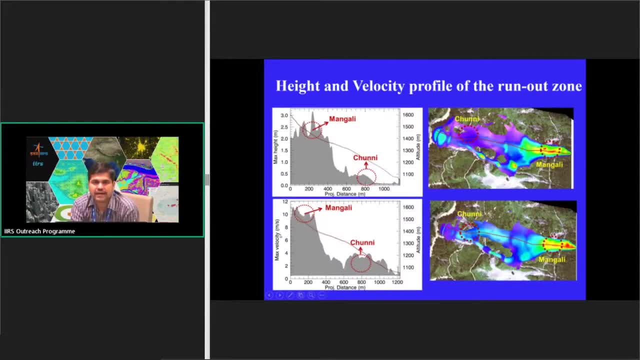 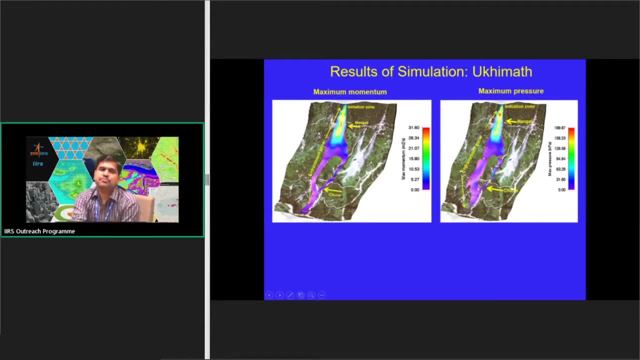 along this line, suppose, and i can, you know, just have a look at how the height or the velocity is varying. maximum momentum and pressure. why momentum is important? because you know the height itself or the velocity itself may not be sufficient at times. because if i want to construct a dam and the dam 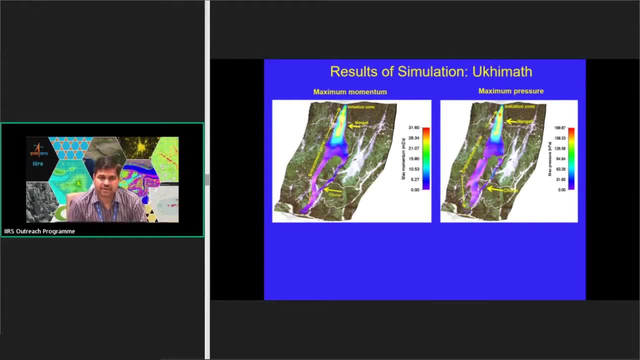 has to be a little bit lower, because if i want to construct a dam and the dam has to be a little bit lower to take the initial thrust of the material that is coming down, so better i calculate the momentum if i take the velocity and the mass all together. so i know the momentum and i can think of you. 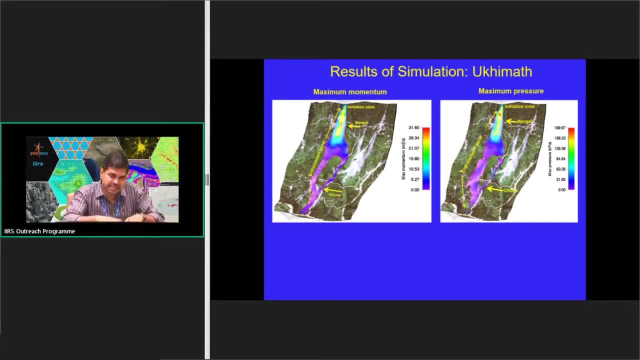 know, implanting a dam. i can think of implanting a dam with a sufficient basement. so dam is a structure like this one, like this the material is coming, like this: if i have a sufficient basement provided to this dam, so it's really strong. so what should the width of this basement 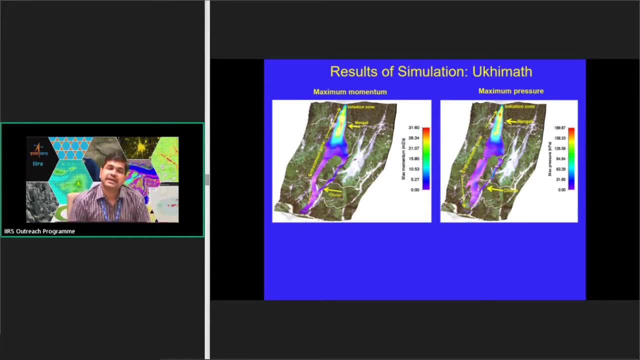 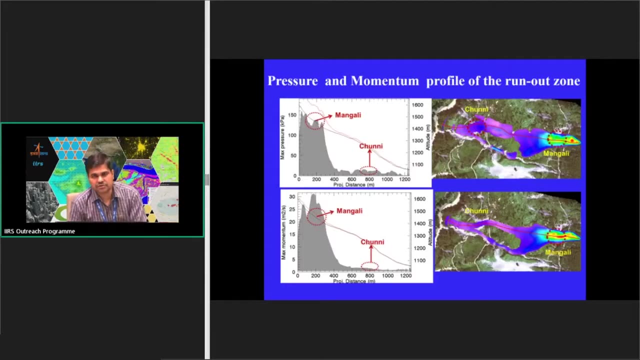 the width of the basement is is dependent upon the momentum the material is coming with. so the momentum is more than the width has to be more so that is the beauty: momentum and maximum pressure also at any spot. you can get to know similar results of profiles also you can get uttrakasi. 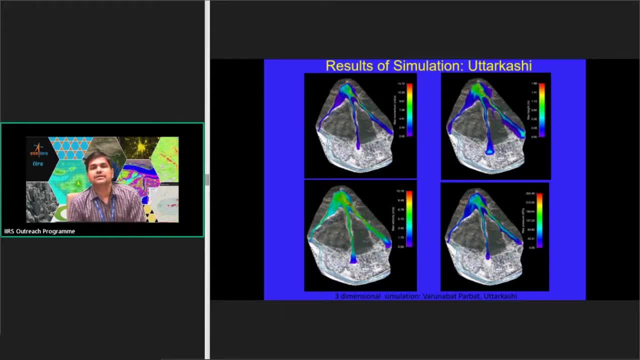 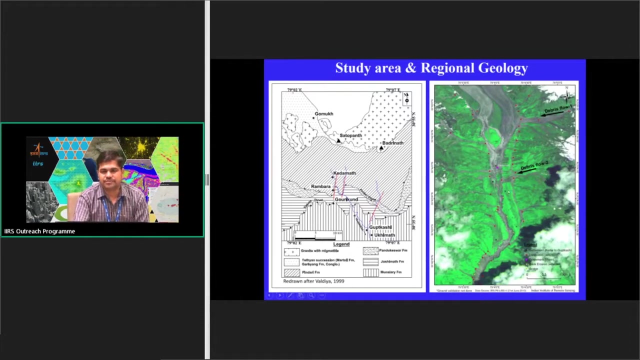 there is, if you remember, there is a trifurcation case- similar results you have got, and please understand that the model has followed the exact torrent, how it happens, naturally. so this is difficult to get but you know, with some exercise you can still model it. profiles and then the kedarnath area. this is a list for image. 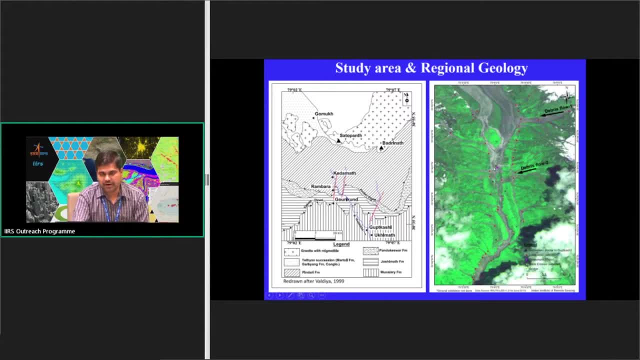 immediate after the flood, and this is where the town is and the material. you know the the your water was available. this is the saraswati river, mandakini river. it was coming like this and then there were, you know, debris flows occurring here, so it basically choked the area. 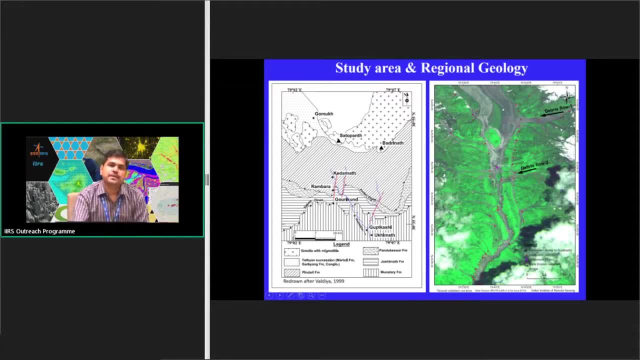 choked, the water shoots and the water was forced to pass through the mid of the town. it has come in one of as a journal paper. if people are interested, they can have a look at it. so if, if the material, sufficient material- is available, we have modeled it. and then i found that there are two blocks here, major debris flow. that basically. 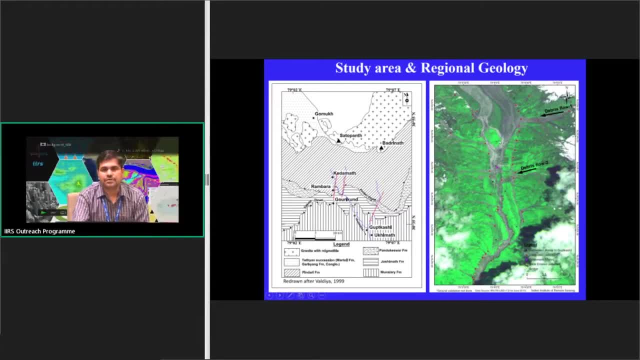 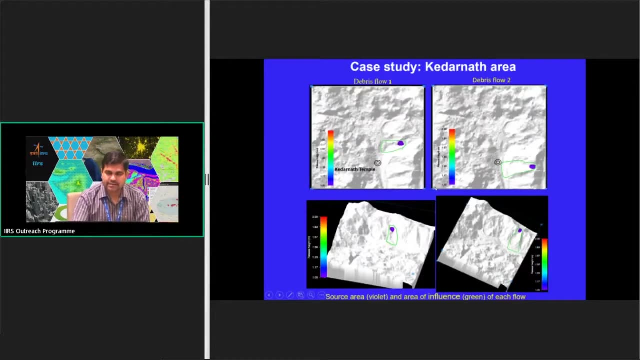 made the material to flow through the city instead of through the town, instead of passing, like this, so that basically created a hubbub. this is the dem of that area, so this is how it looks like. this is the temple and this is how the model- uh sorry, the on the dm, the source area, um, lies, like this: 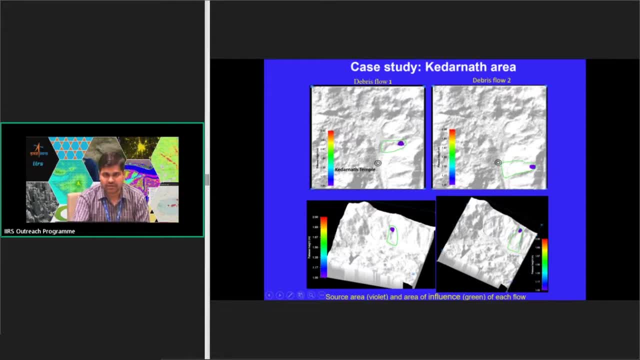 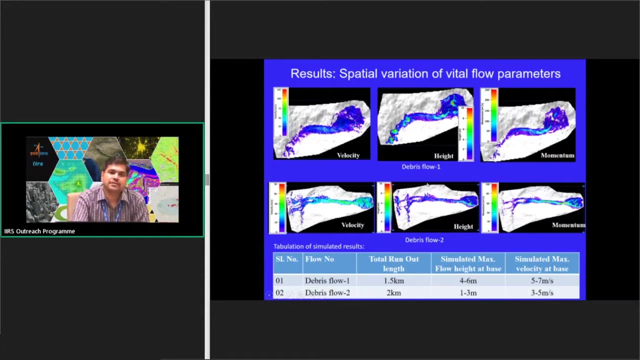 this is the source area. this location is the temple location. so one debris flow we have taken above the upstream of the temple, another slightly downstream, and this is the result. the result, basically told, tells that the velocity, height and momentum, how they are varying, or flow one and flow. 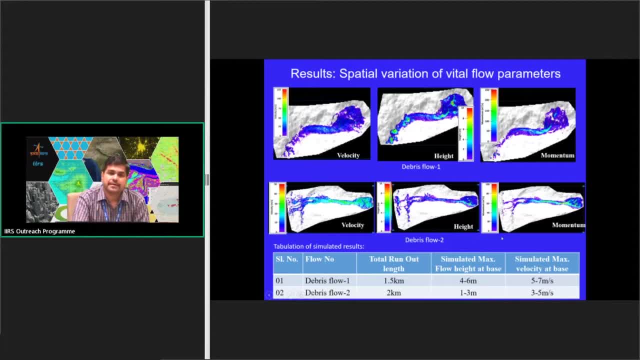 two. please note down their velocity: five to seven meter per second for flow one. there's upstream one and uh, the total run out was 1.5 kilometer. it was coming from the north one, and then total maximum height is four to six meters- six meter, mind it. 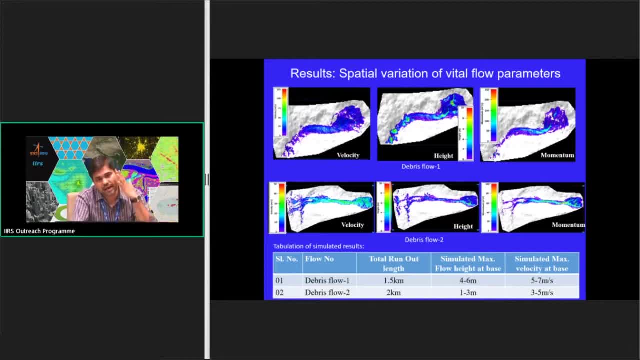 so the six meter height is quite enormous. to no, at least partially block the saraswati river or mandakini river, so that the water- available water- was forced to make its path at least resistant path through the town itself. that is how the town got washed away. 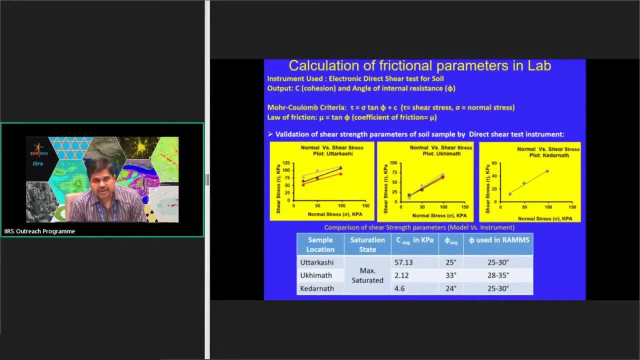 then sort of have postulated in that paper. so i was telling about how to validate this because some input parameters- if you remember mu and xi, they were g-engine properties parameters and that we can get it back from, also from the lab specimen also have checked that you. 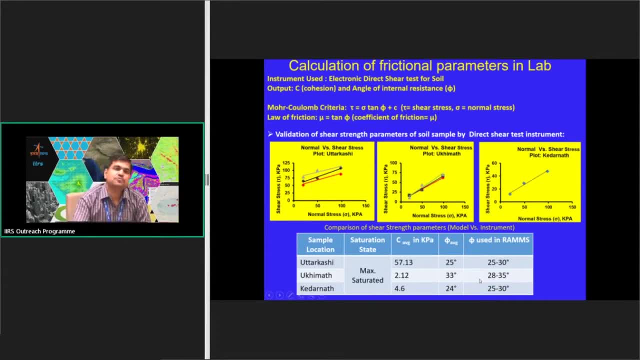 know, uh, the the parameters, input parameters that we have given, uh, as input to the model, and what we got from the field. we have tried to model them and then then we found that they are, you know, quite at par, they're, they're almost similar. so that basically indicates that our models are. 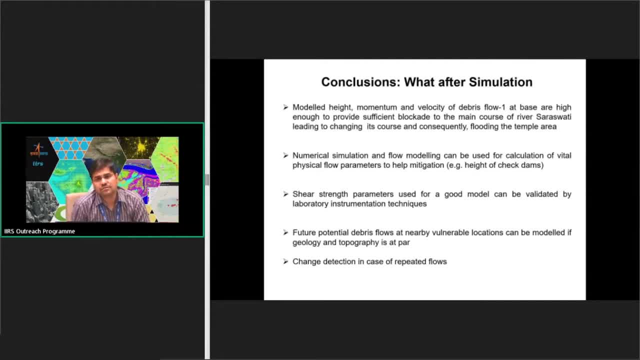 authentic. so what are the what after the simulation? what do i do with this model? height, momentum and velocity of the flow. suppose, in case of db flow, one in they were sufficient enough to provide sufficient blockade to the main course of the river. that's changing its course and 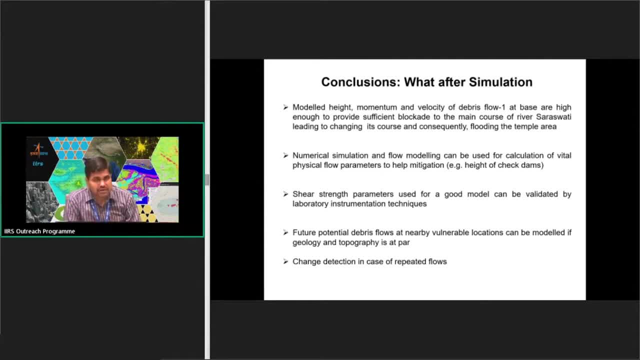 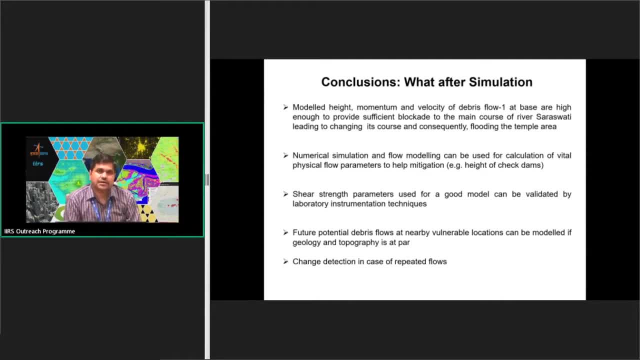 mitigation. so height of the check dams etc can be, you know, modeled uh, can be, you know, height of the dam can be fixed by the model inputs. model outputs, shear strength parameters, specially of a good model, can be validated by laboratory instrumentation techniques, the xi and mu1, that can be, you know, verified from the field, collected samples and the future. 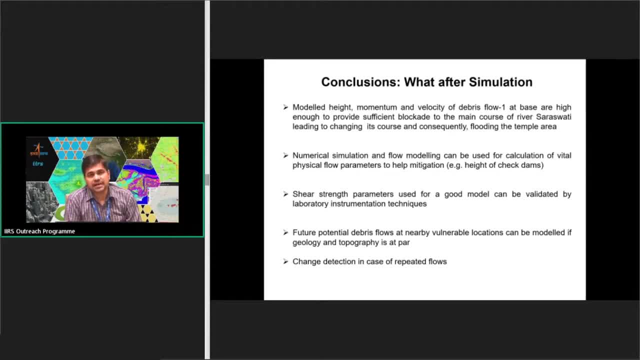 potential models, because many of the time, many times, it happens that big landslide, once it has happened, it will keep on happening for decades. it doesn't stop as such. so if it is keep on happening, uh, every in every monsoon, suppose. so what today it is? you know the shape. 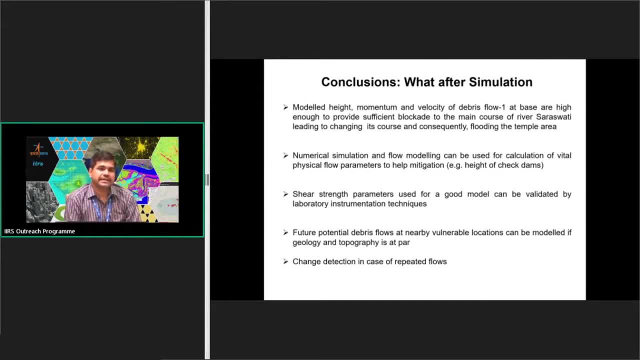 is like that: from a satellite image you can get to know, from field also you can check and suppose next monsoon. you think that this much you know beyond today's area is this and beyond that the next monsoon it's going to, so this additional material is going also to going to fall down. 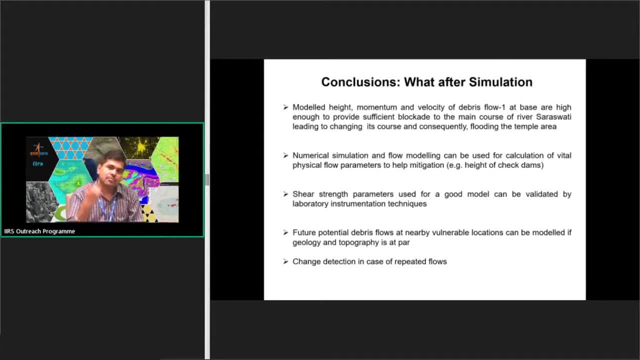 so if that material is available for the landslide to slide down, my model can tell you that what should be. the more uh run out path, more area it will cover and obviously the variation of four parameters. so that can you know. you can use it for a futuristic model also. and the things become 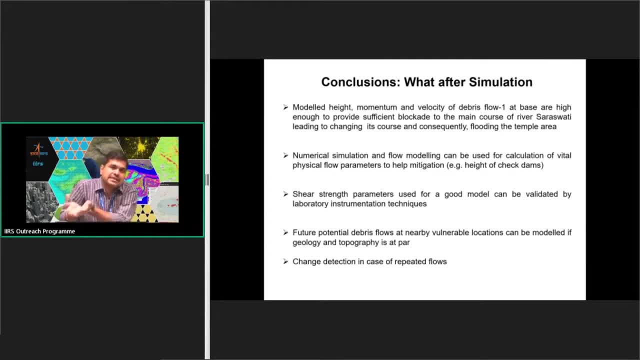 quite easy, uh, for suppose one area it is happening and the adjacent area also it has started. so with the same gene engineering property, same geology. if it is continuing, i can give my same inputs also there, because geology is not going to change in 5, 10 kilometers. so if it happens, so it's very